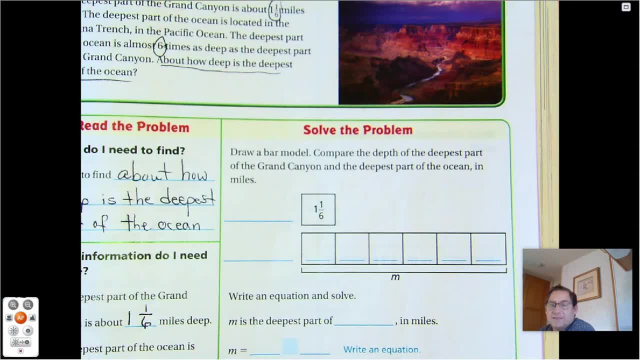 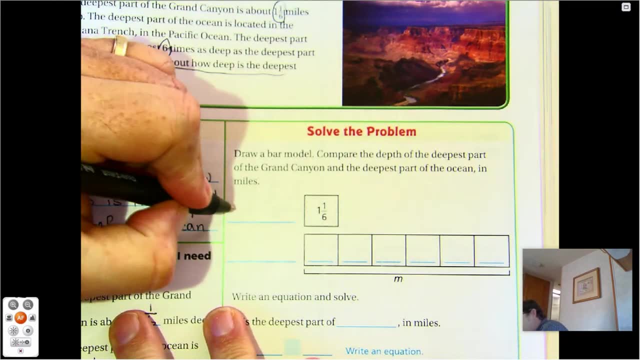 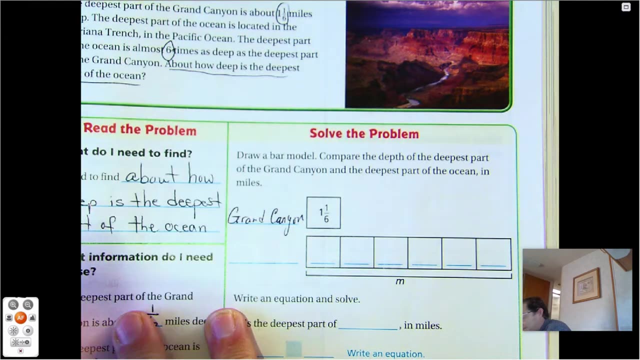 It says: draw a bar model and compare the depth of the deepest part of the Grand Canyon and the deepest part of the ocean in miles. So one and one-sixth, that refers to the Grand Canyon And the deepest part of the ocean. we can say Mariana Trench or we can just write ocean. 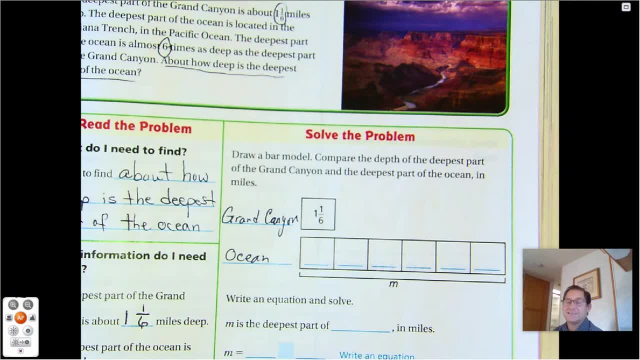 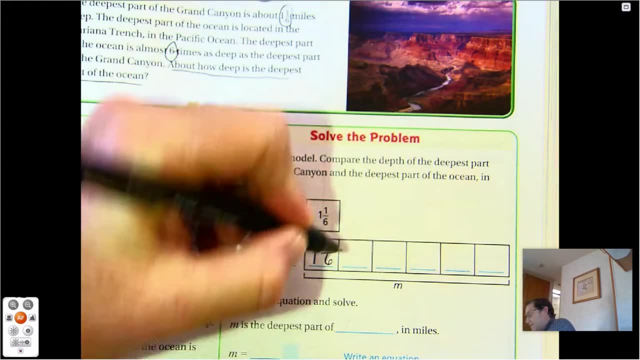 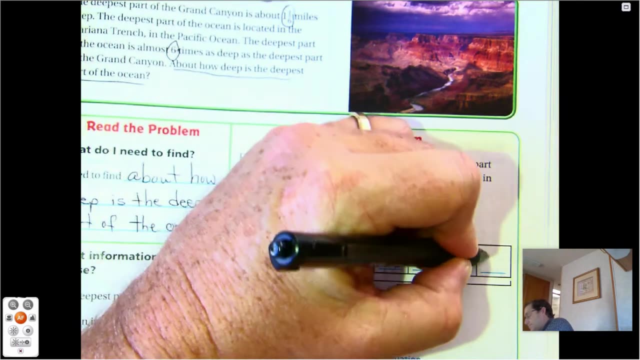 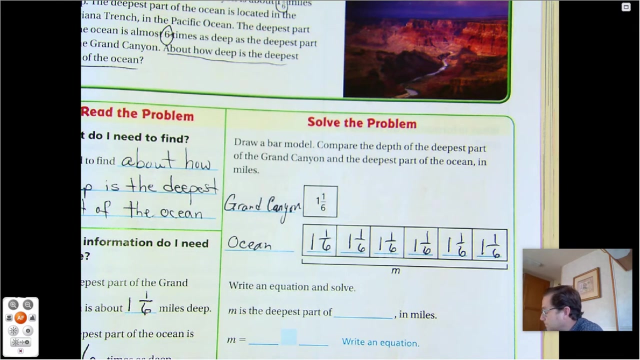 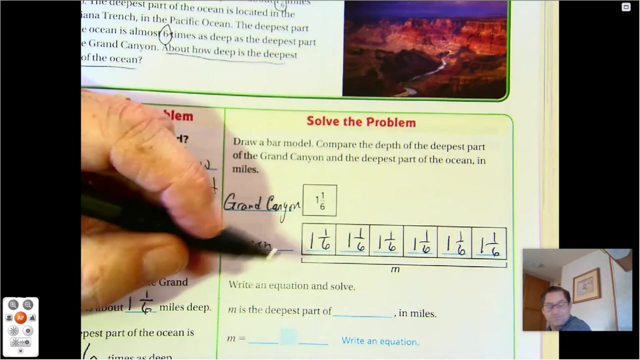 Okay, is six times as much, So each part is going to be one and one-sixth times Okay. so we have six, one and one-sixth, So write an equation and solve. M is the deepest part of the ocean in miles. 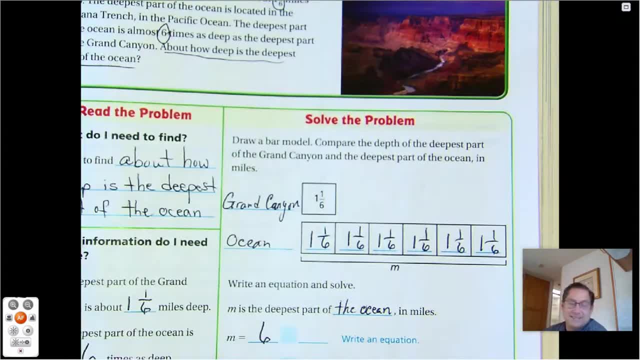 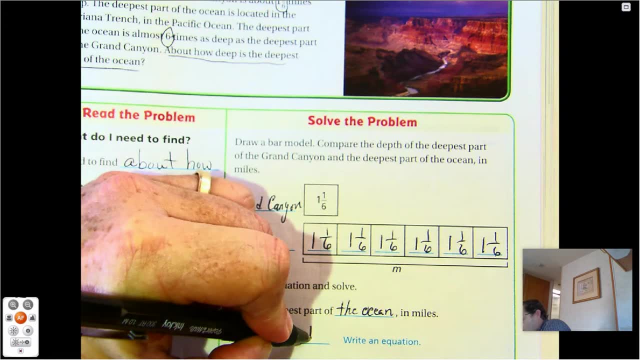 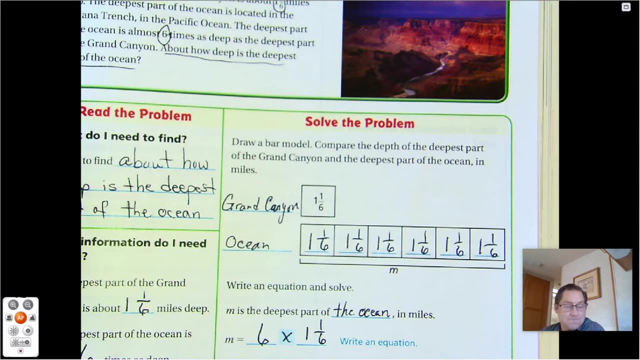 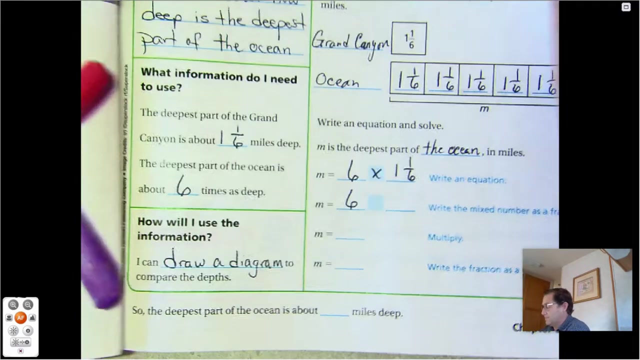 So M equals six. We have six parts in that problem, Times one and one-sixth, Because it said the ocean was six times as deep. So we're going to leave the six. Write the number: the one and one-sixth, the mixed number as a fraction. 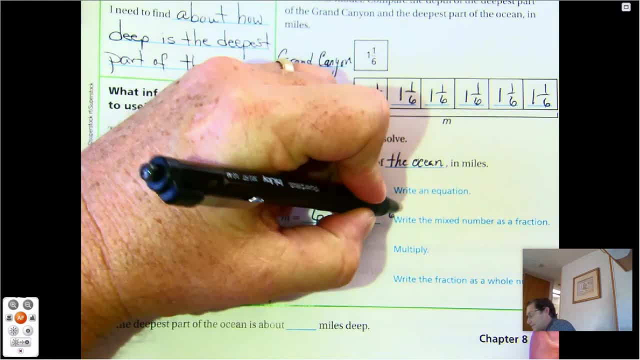 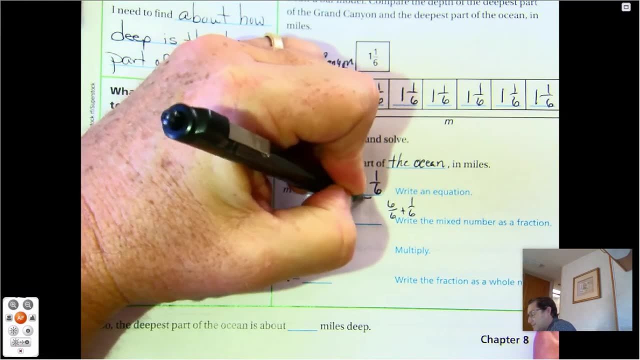 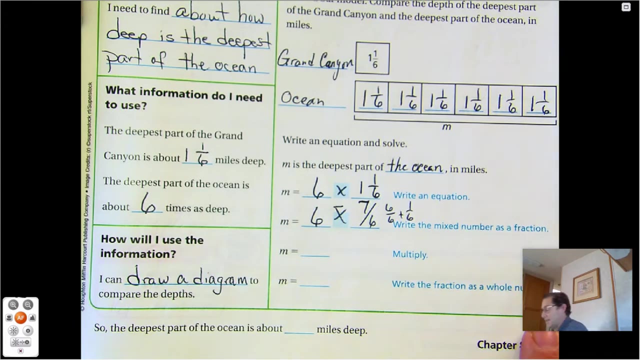 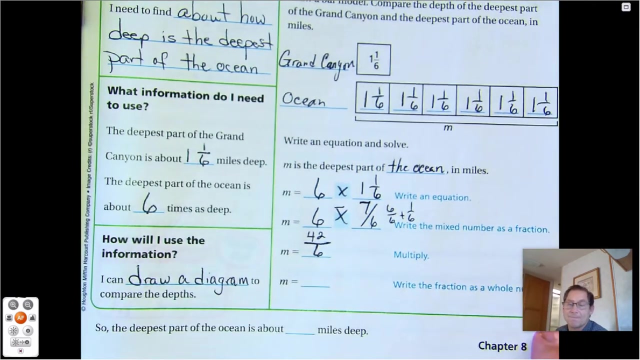 Well, we know that one is worth six-sixths plus the one-sixth, So that's seven-sixths, All right, so how much is six-sixths? How much is six times seven-sixths? Six times seven is forty-two-sixths. 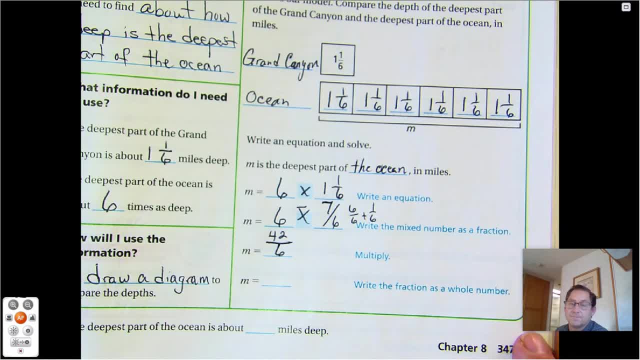 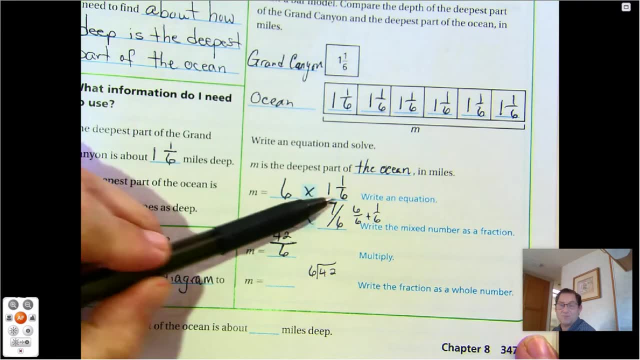 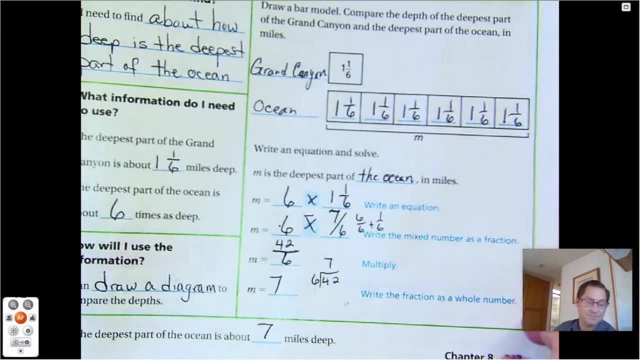 So now write the fraction as a whole number. What is forty-two divided by six? Well, if six times seven was forty-two, then forty-two divided by six has got to be seven. So it's about seven miles deep, Which is really deep when you think about it. 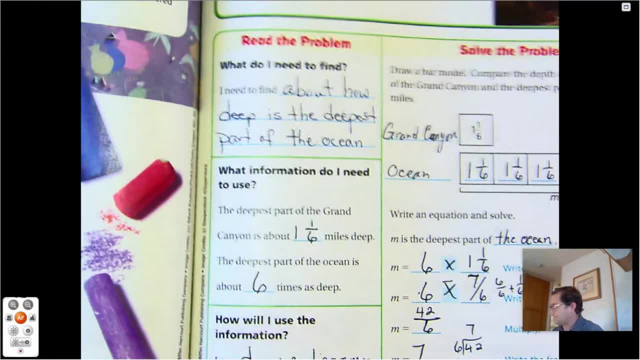 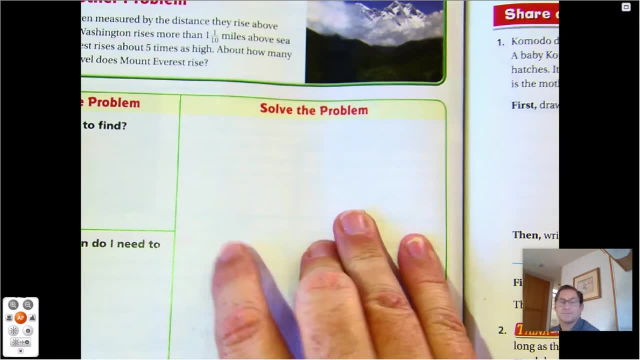 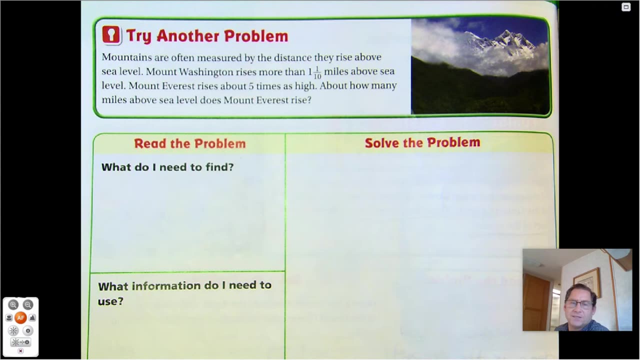 All right, try another problem. We're on page 348.. Mountains are often measured by the distance they rise above sea level. Mount Washington rises more than one and one-tenth miles above sea level. Mount Everest rises about ten miles above sea level. 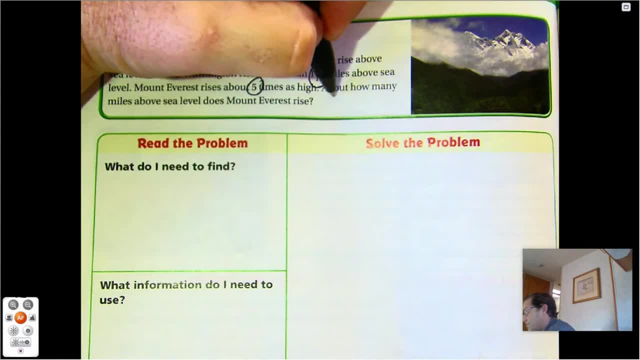 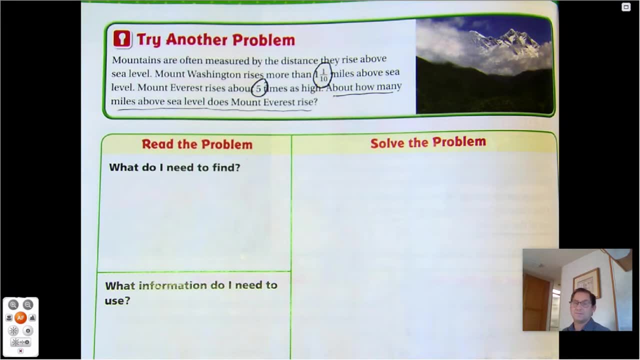 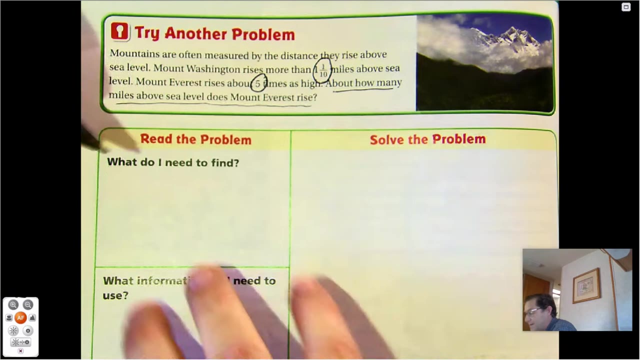 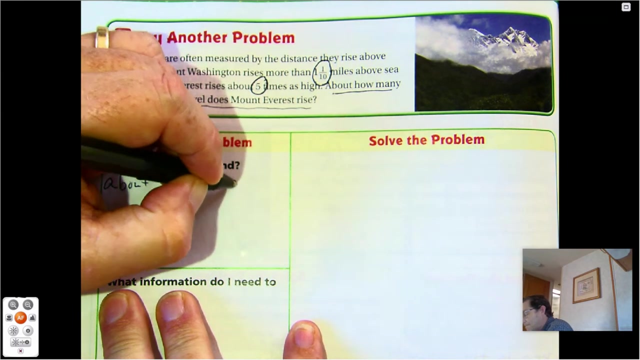 Five times as high. About how many miles above sea level does Mount Everest rise? So this is the same question as the ocean being deeper than the Grand Canyon, except we're referring to mountains. So what do I need to find About how many miles above sea level? 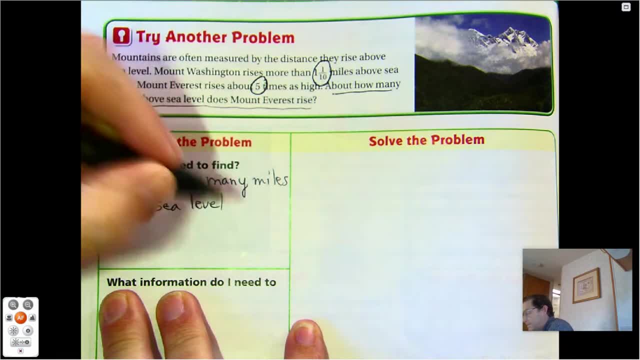 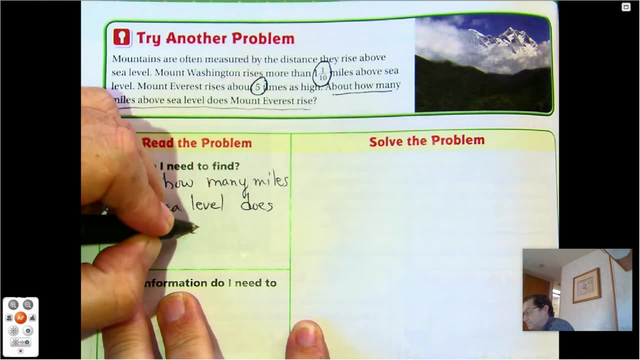 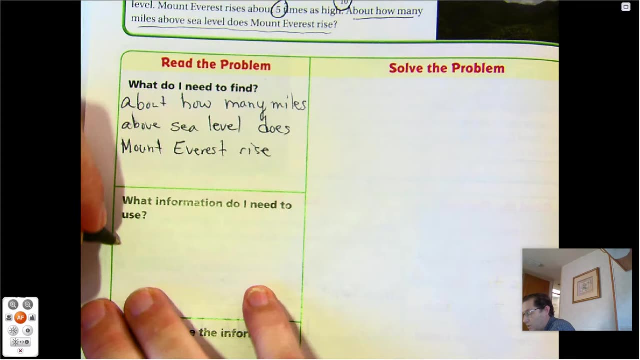 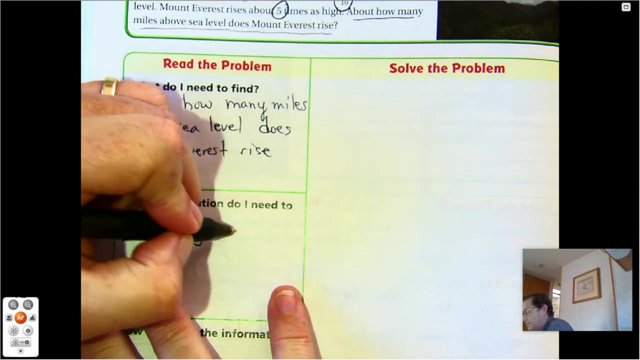 I need to find information on Mount Everest. Does Mount Everest rise All right? What information do I need? Well, I need to know that Mount Washington is one and one-tenth miles above sea level And Mount Everest is six miles above sea level. 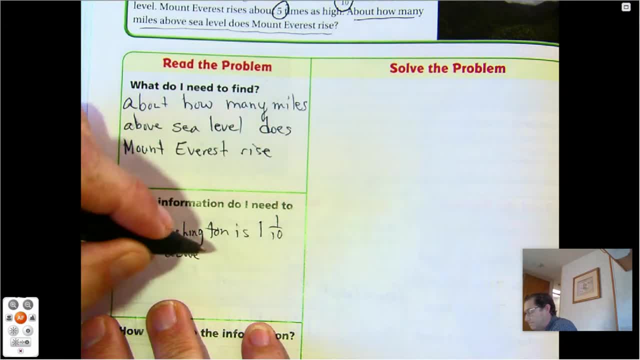 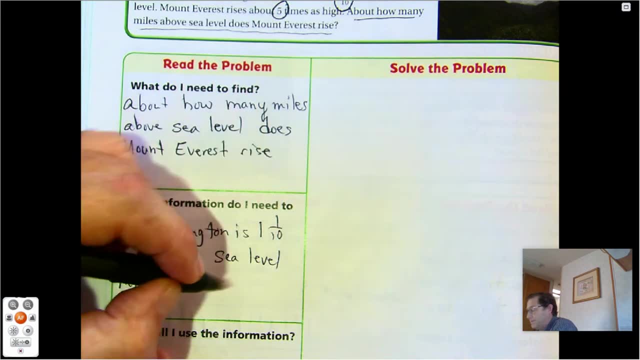 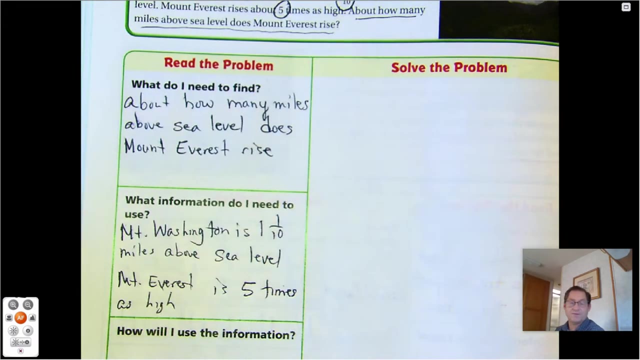 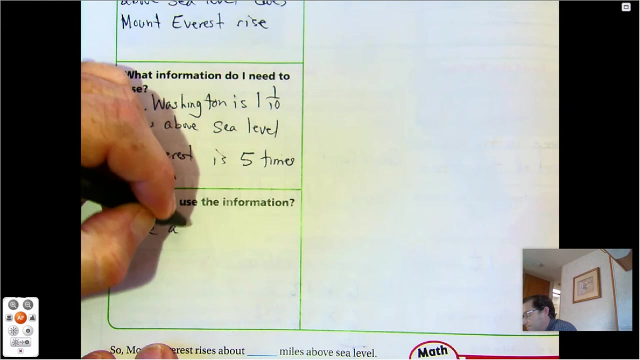 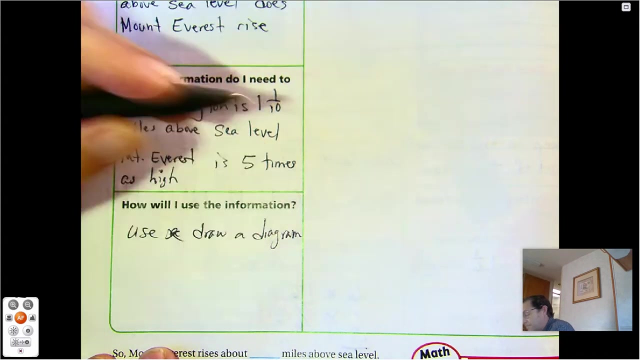 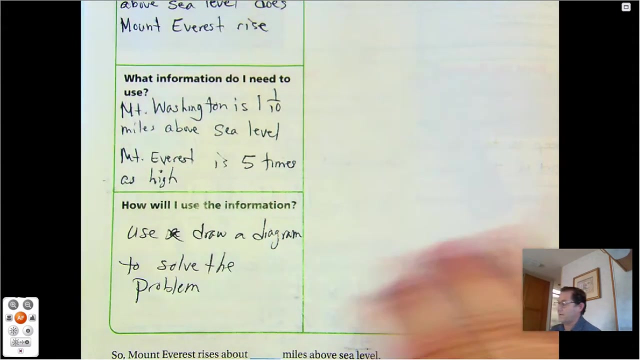 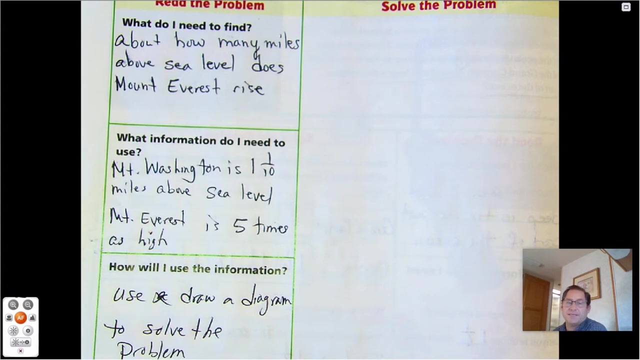 miles above sea level and that Mount Everest is five times as high. how will I use the information? well, we're going to use the same model that we did in the last one, so use a diagram, use, draw a diagram to solve the problem. okay, so let's review. what do I need to find about how many miles above sea? 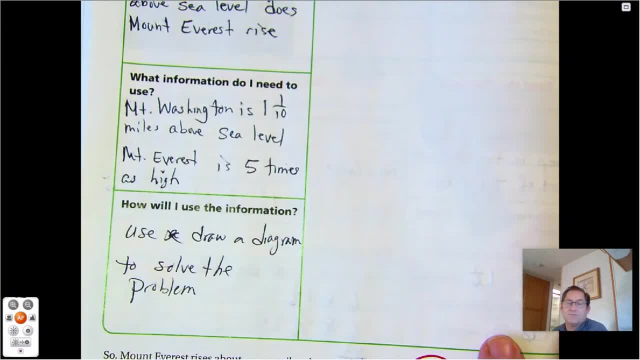 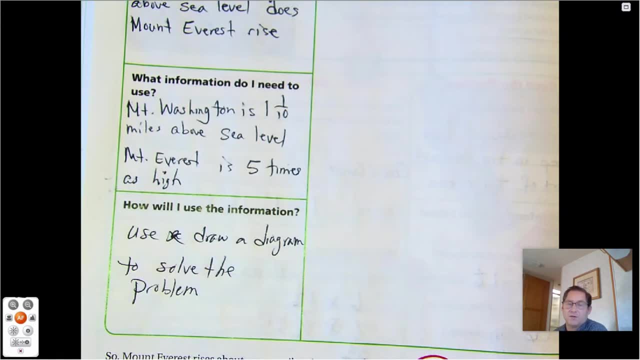 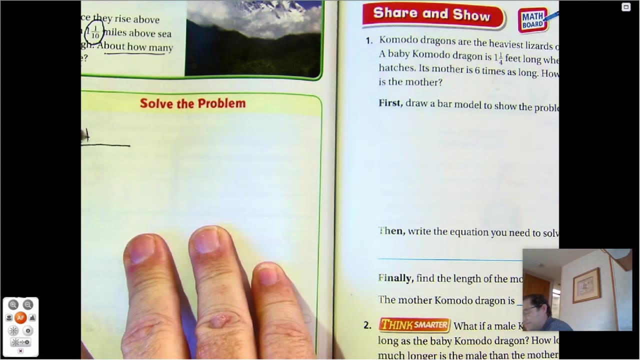 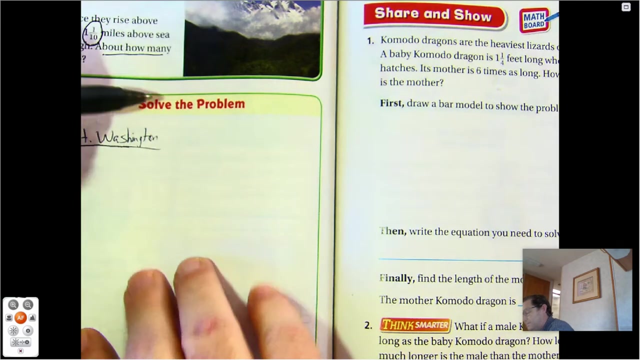 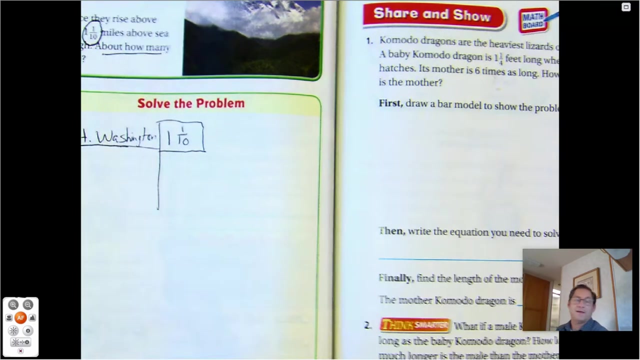 level does Mount Everest rise? Mount Washington is one and one and one-tenth miles above sea level. Mount Everest is five times as high and we're going to draw a picture to show that we're going to start with Mount Washington and we know Mount Washington is one and one-tenth miles above sea level. Mount 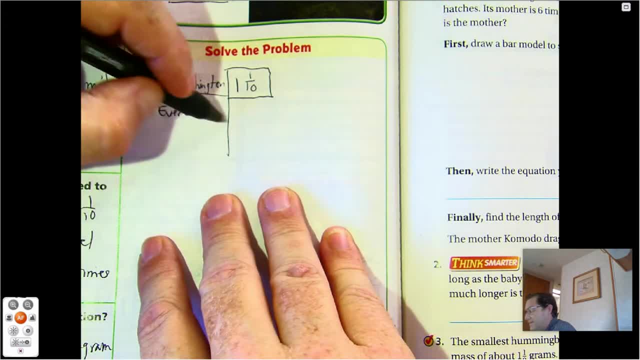 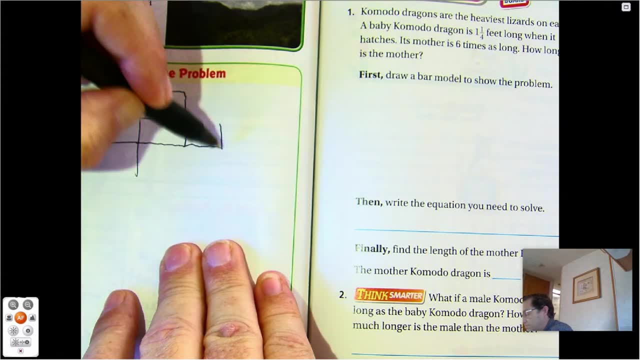 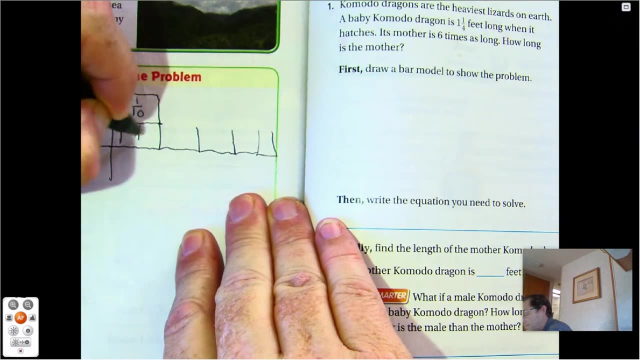 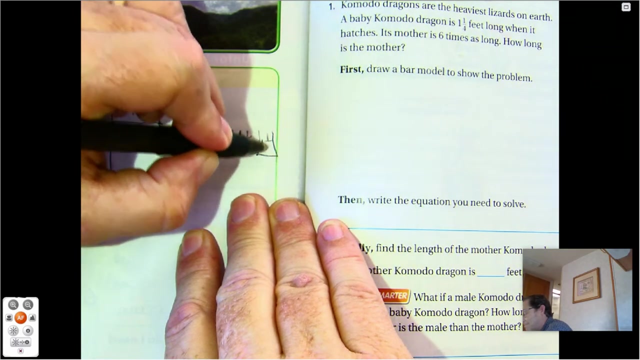 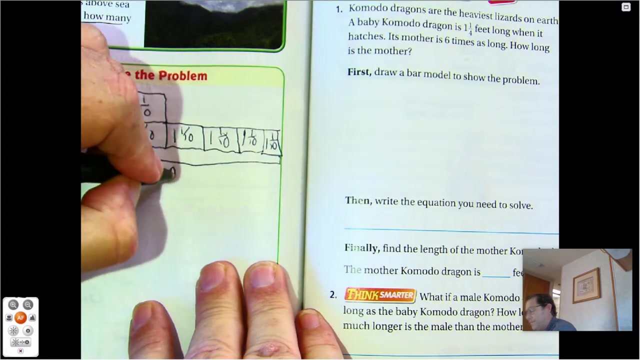 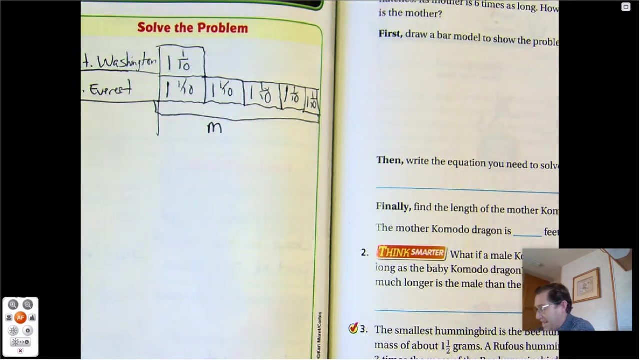 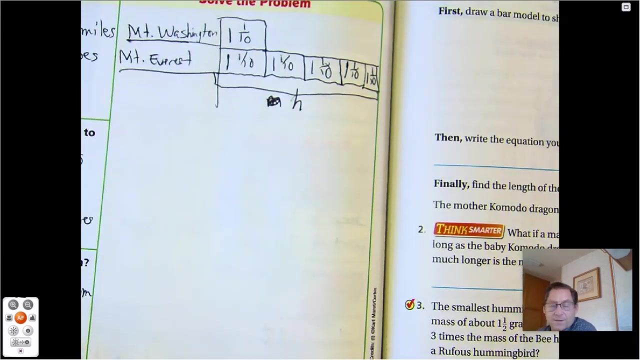 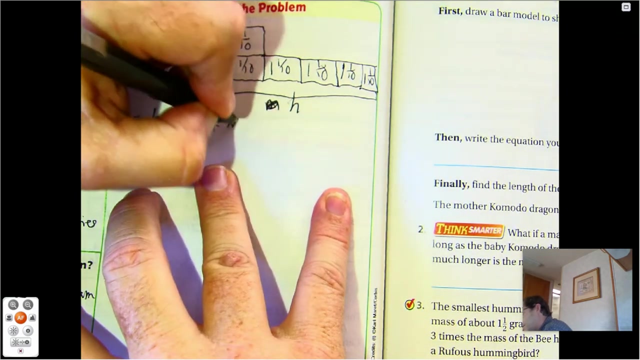 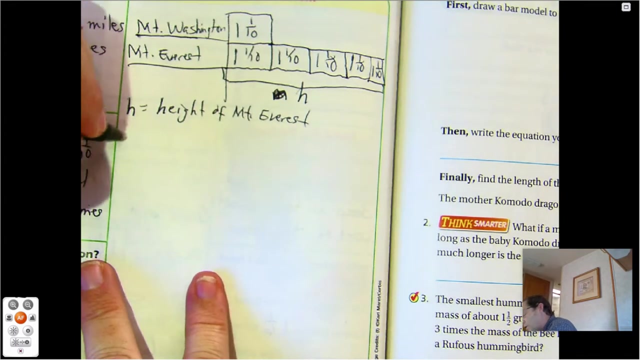 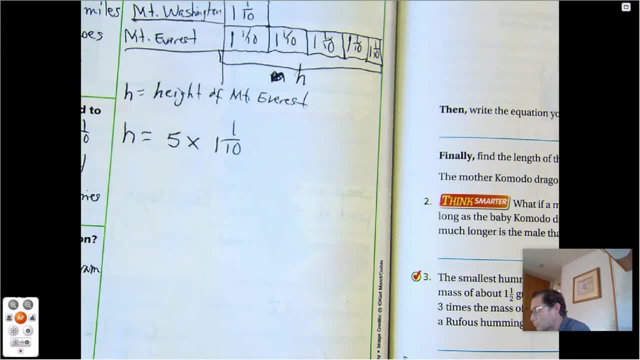 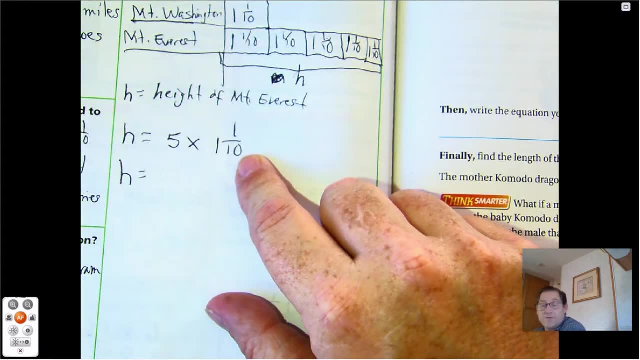 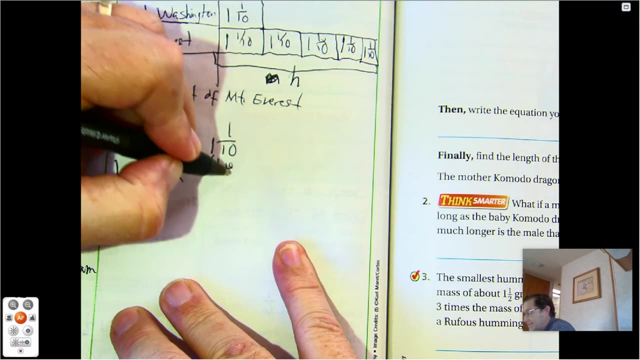 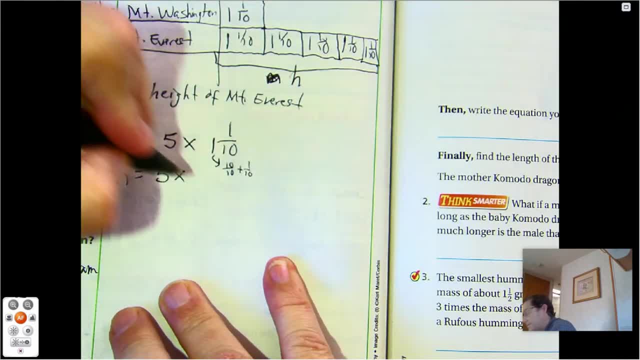 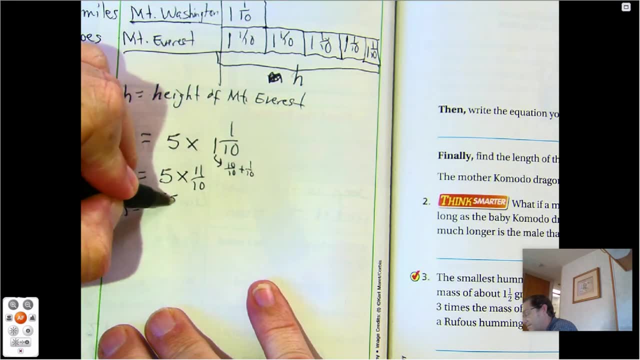 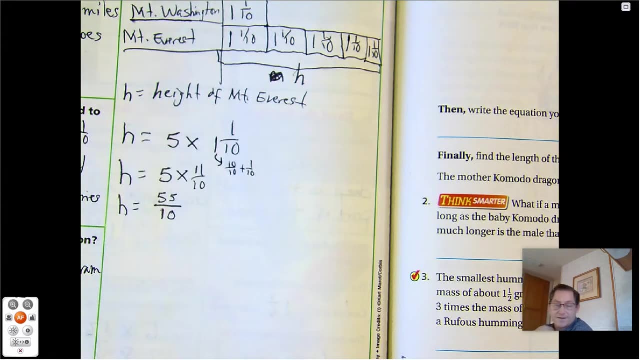 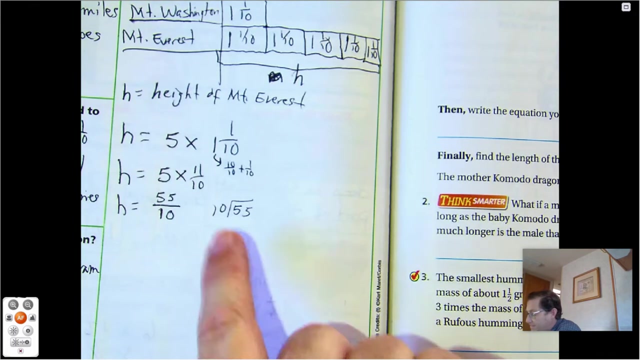 tenths. So 10 tenths plus 1 tenth is 11 tenths. So what is h? equal 5 times 11 is 55 tenths. Now let's change that into a mixed number. Okay, So 55 divided by 10.. I can't share the 5 tens into 10 groups equally, but I can share 55. 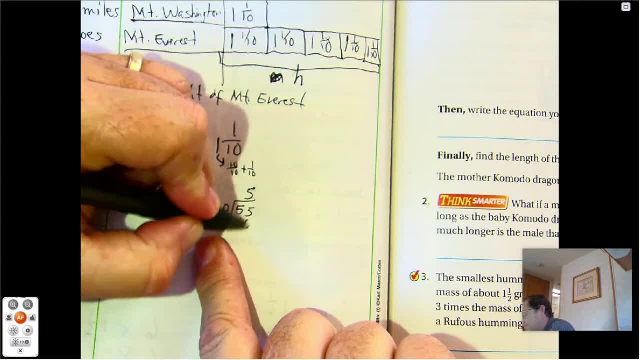 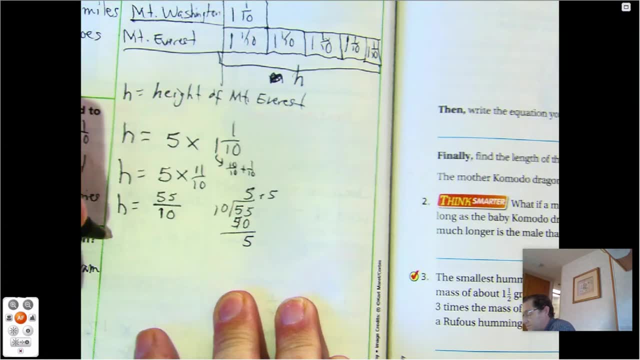 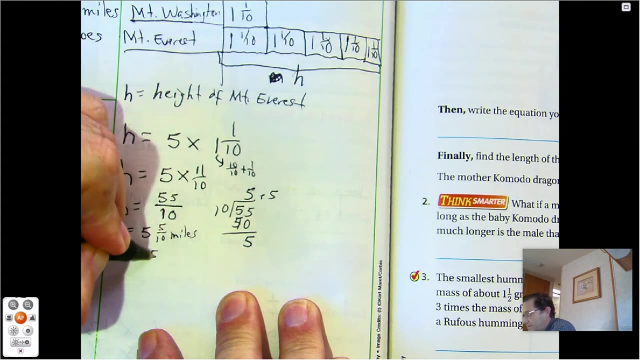 ones equally into 10 groups 5 times. So 5 times 10 is 50 with a remainder of 5.. So 5 remainder 5.. So the height is 5 and 5 tenths miles, Or 5 and 1 half miles. 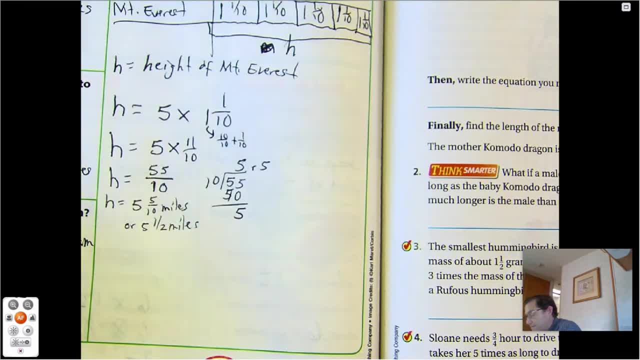 So Mount Everest rises about 5 and 5 tenths, or 5 and 1 half miles above sea level. How did drawing a diagram help you solve the problem? I could see that Mount Everest had 5, 1 and 1 tenths in it. 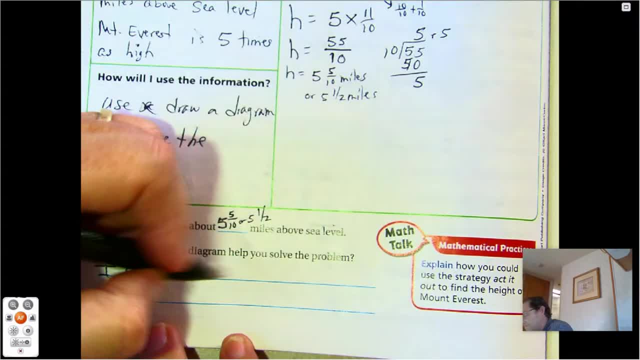 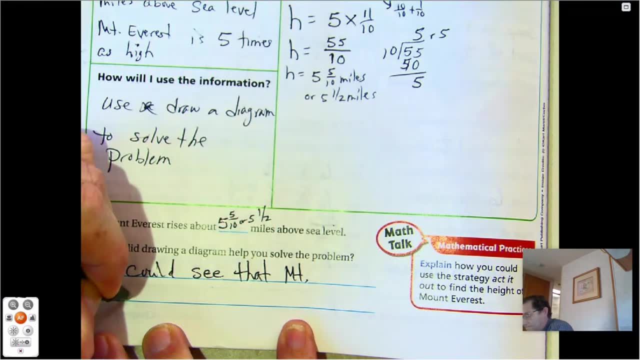 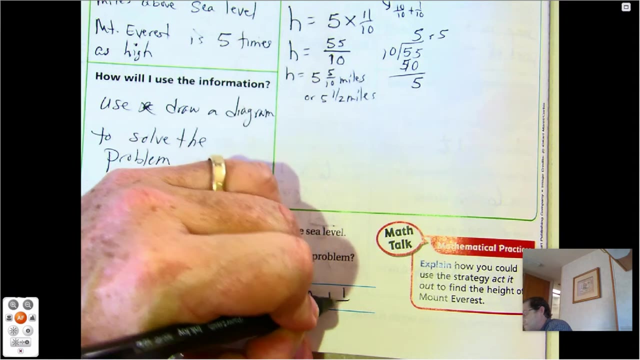 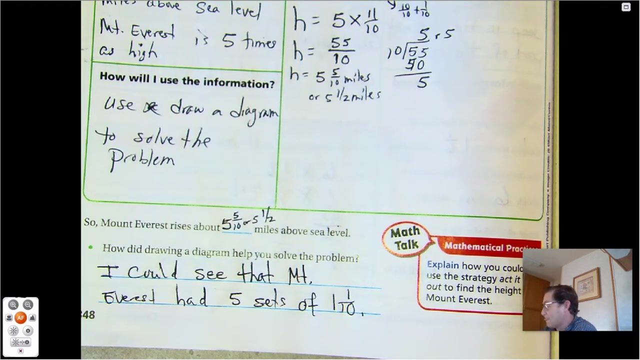 Make a question. Hahaha, I did that for you. Okay, Now I can see that Mount Everest had 5 sets of 1 and 1 tenths. Alright, Page 349.. As she cannot see, subject will move further Number 1.. 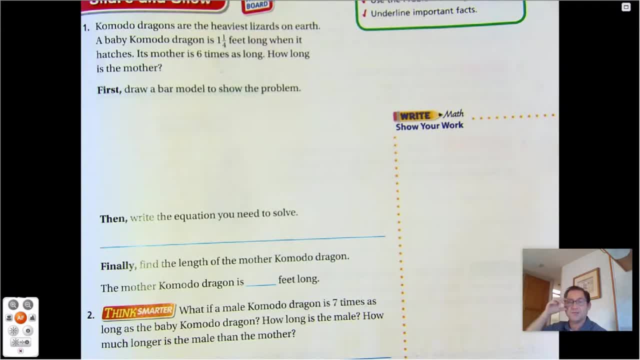 Number 1اح. Number 2, is 127.. Number 1 in six. Number 2, is 2,th, Three tenths and one tenths of the one tenth in it. Komodo dragons are the heaviest lizards on earth. 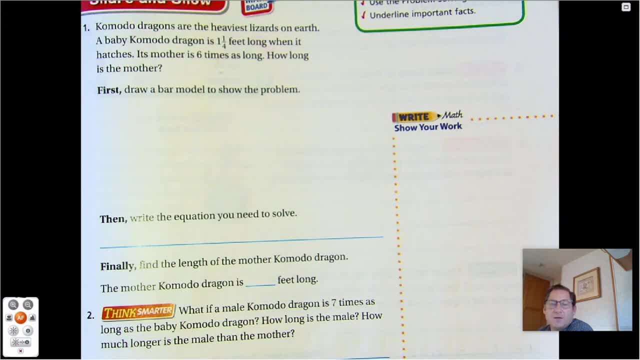 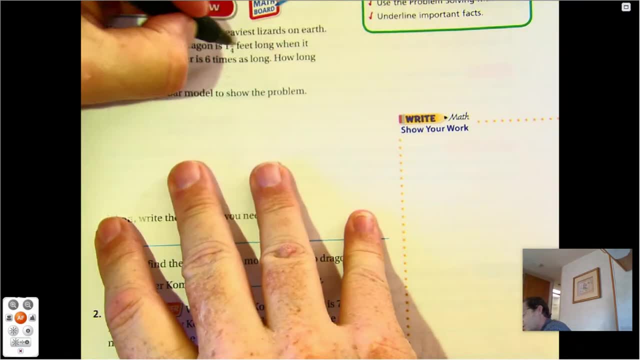 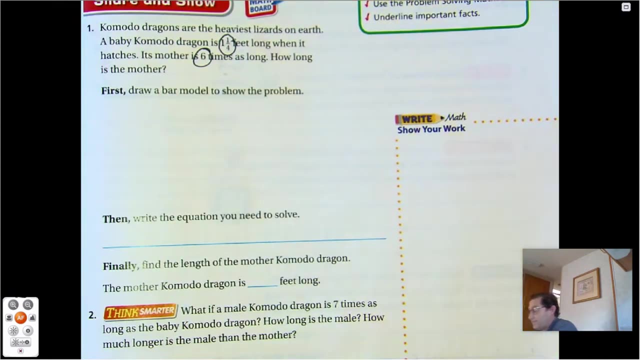 A baby Komodo dragon is one and one-fourth feet long when it hatches. Its mother is six times as long. How long is the mother? Six times as long, Wow, Okay, first draw a bar model. Okay, so we're. 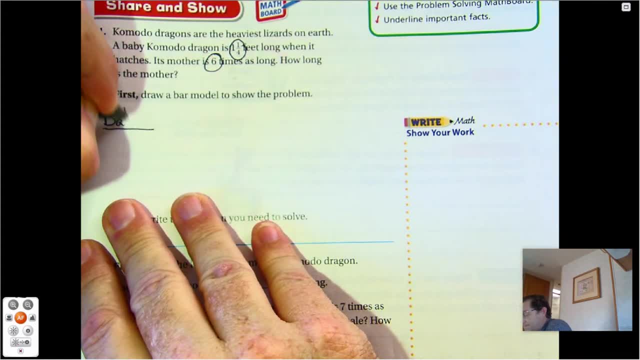 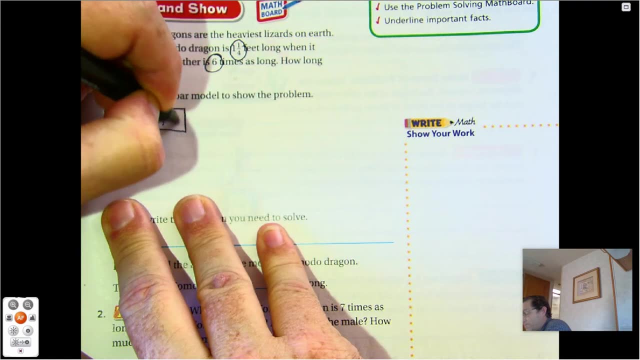 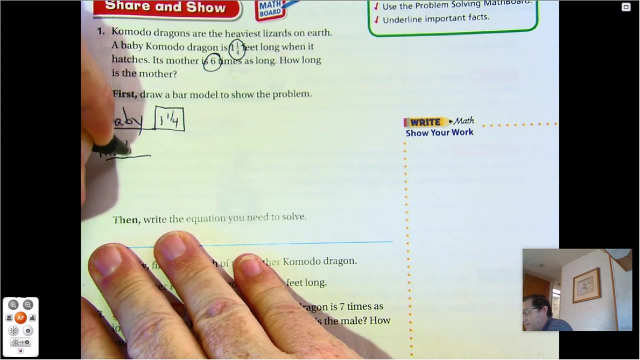 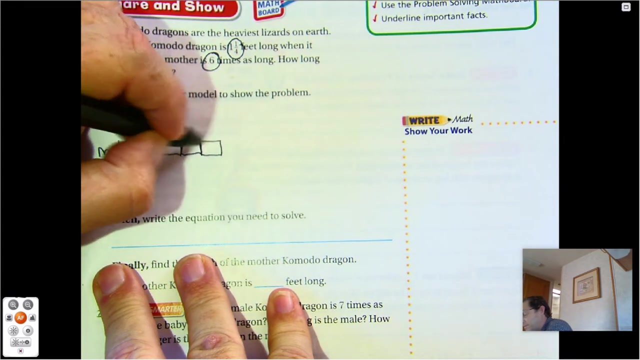 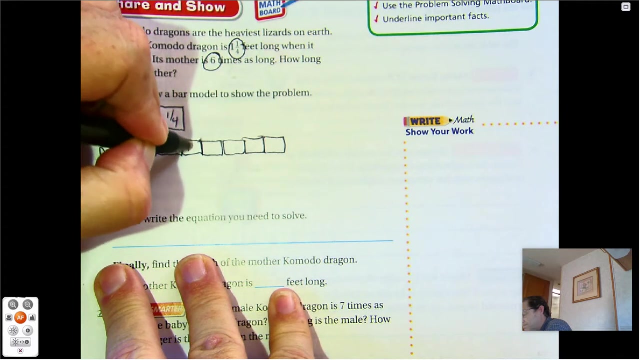 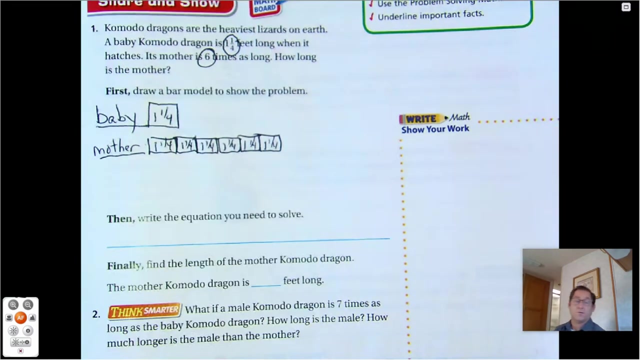 going to start with the smaller one. So we're going to say baby, And the baby is one and one-fourth feet. The mother is six times as much. So how many? one and one-fourths Six. Okay, now we're going to write an equation. 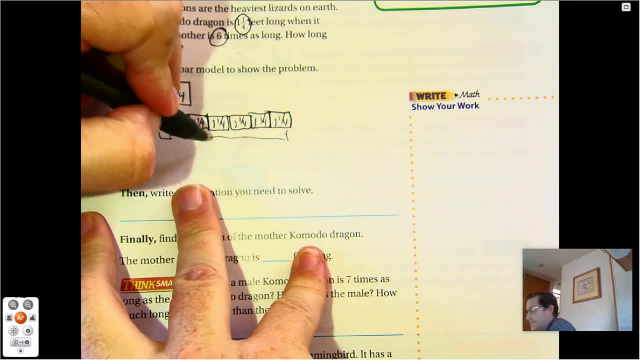 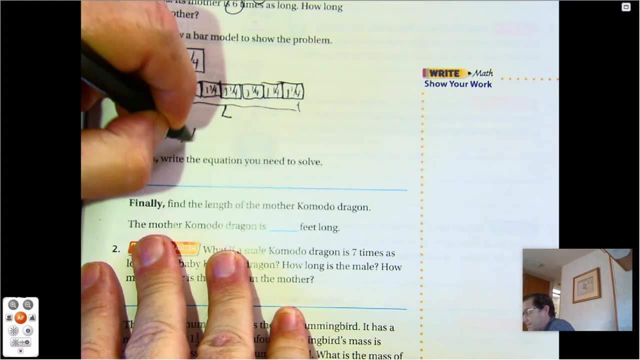 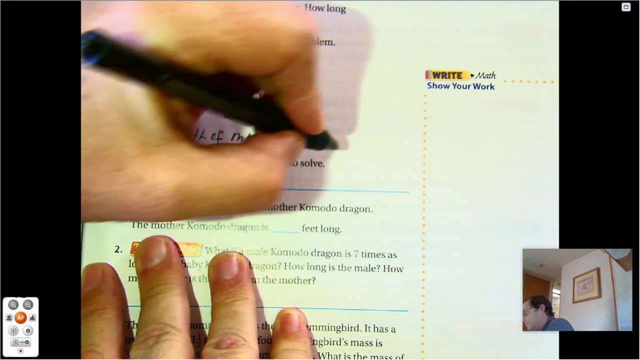 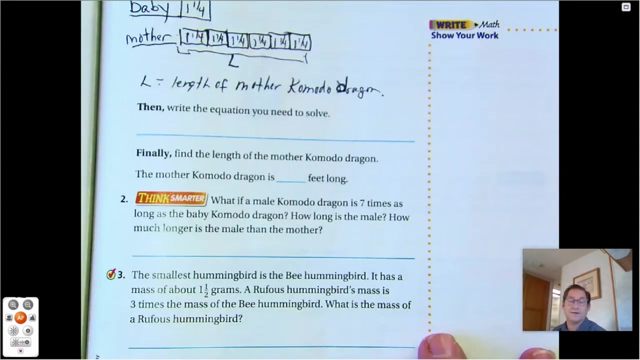 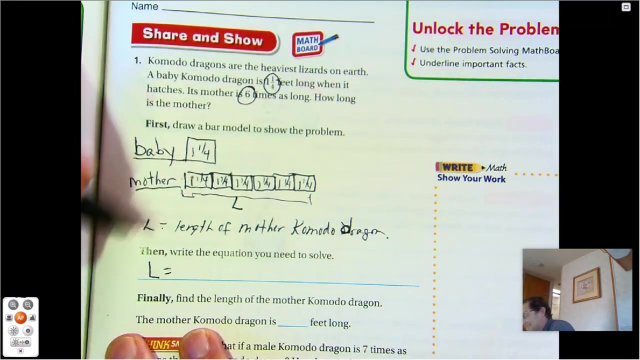 So we could say: this is the. we can call that L for the length. So L equals length of mother Komodo dragon. Okay, Komodo dragon, Write the equation. So L, the length of the Komodo dragon equals six times one and one-fourth. 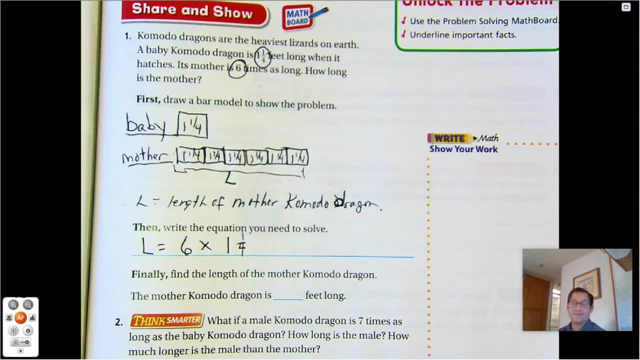 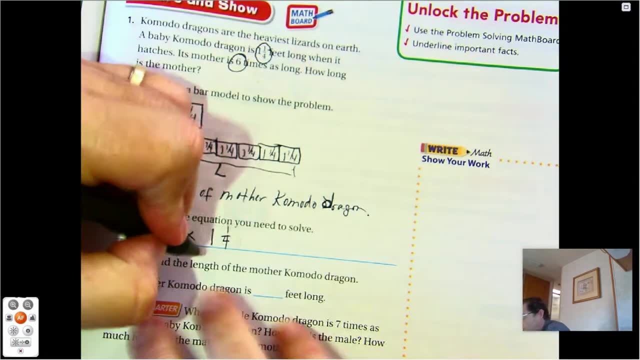 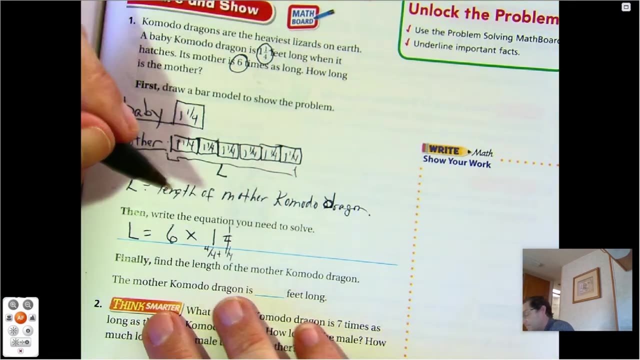 So six times the baby's length, Find the length of the mother Komodo dragon. Well, so we're going to change one and one-fourth To four-fourths plus one-fourth. Okay, four-fourths is one. So now we have L equals six times five-fourths. 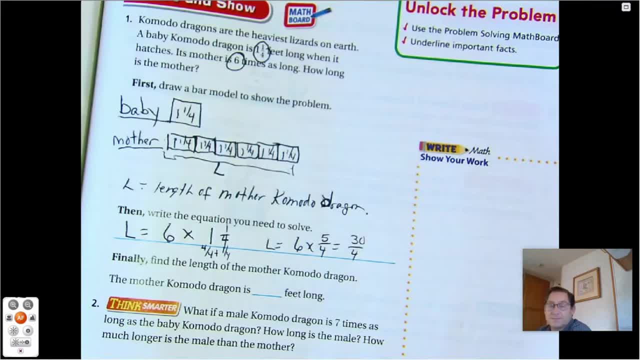 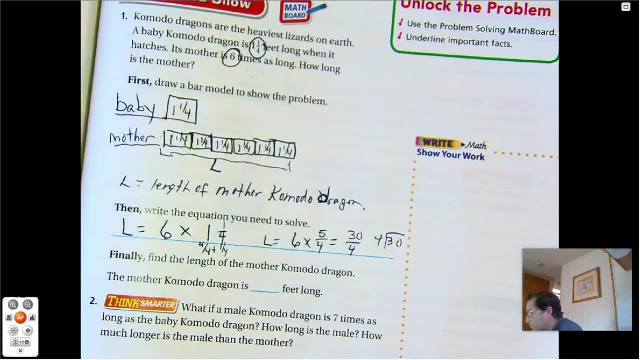 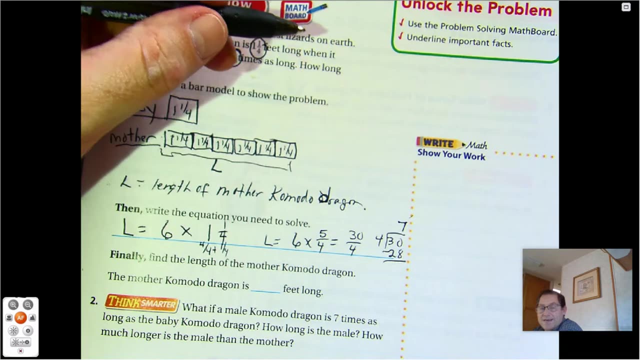 Six times five is thirty, So we have thirty-fourths. Change it back into a mixed number by dividing Thirty. divided by four. Seven times four is twenty-eight, leaving me two ones. I can't share those equally, so I have a remainder of two. 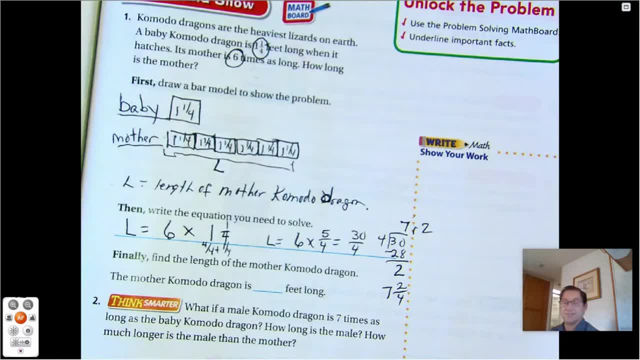 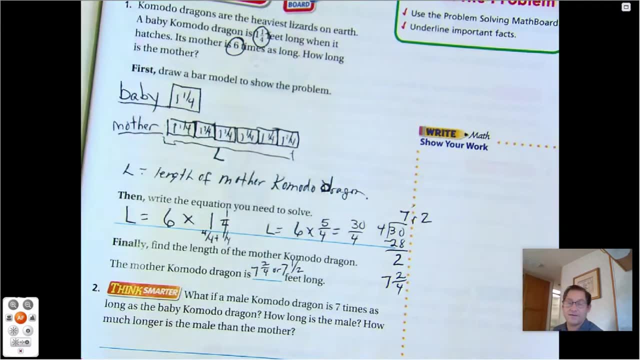 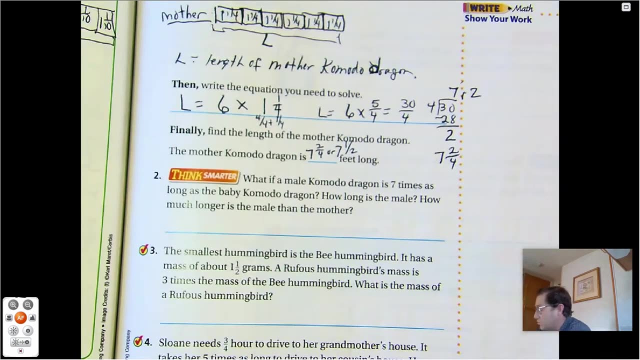 So the Komodo mother Komodo dragon is seven and two-fourths feet, Four-seven and one-half feet long. I see that four two is four-half of four. All right. well, what if a male Komodo dragon is seven times as long as the baby Komodo dragon? 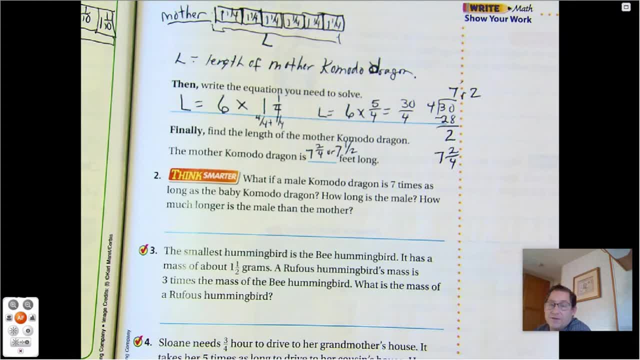 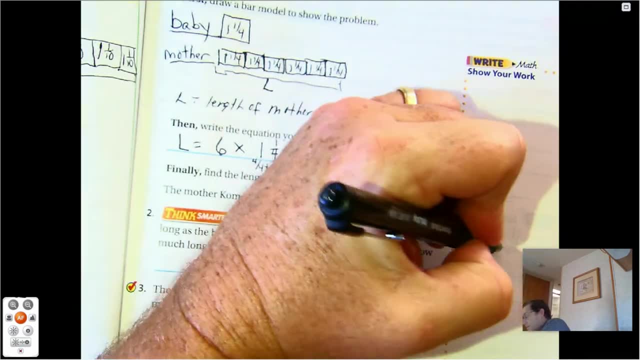 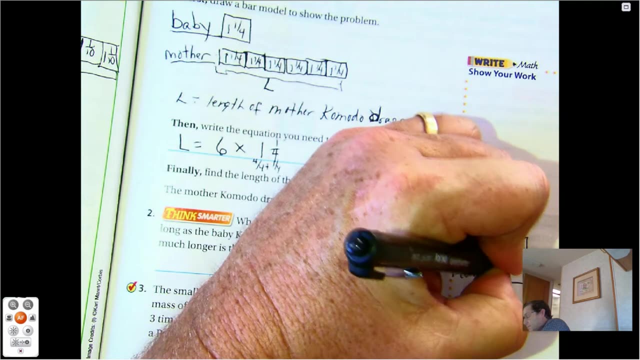 How long is the male? How much longer is the male than the mother? Well, so if we're going to draw a picture for that, one again we'd have: the baby would be one and one-fourth And the male would be seven times as much. So this time we're going to have seven boxes. 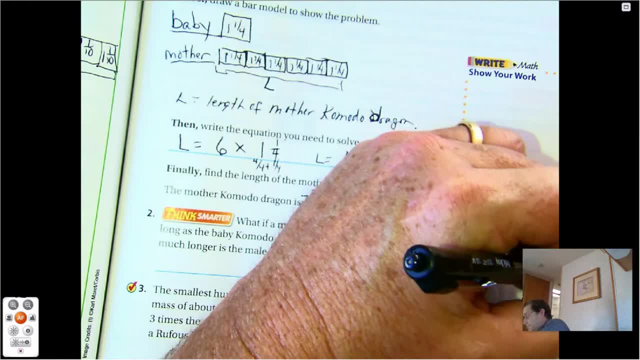 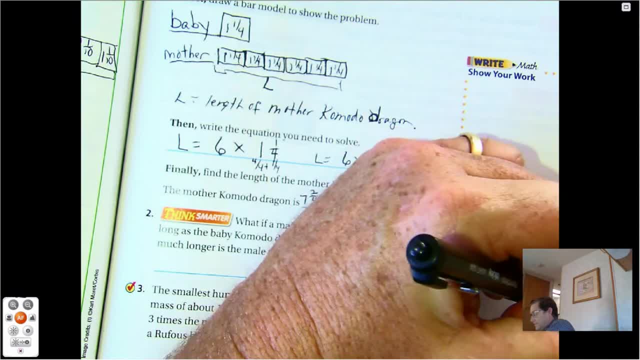 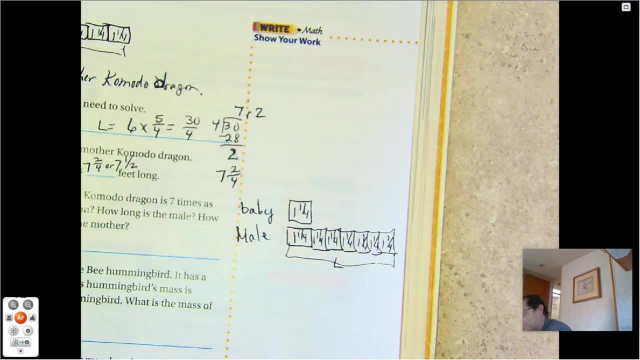 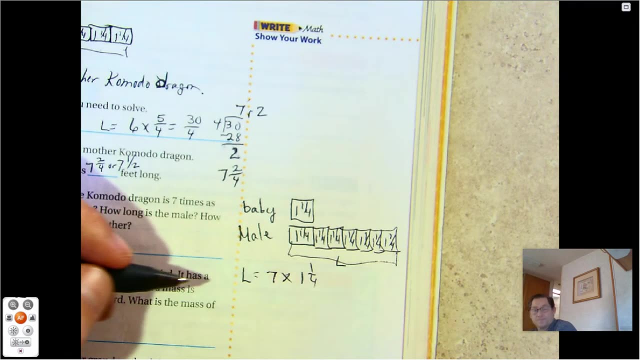 Okay, so our equation: We're going to go ahead and let L again represent the length of the male Komodo dragon, And so we'll have: L equals seven times one and one-fourth. We're going to change the one and one-fourth into a mixed, into an improper. 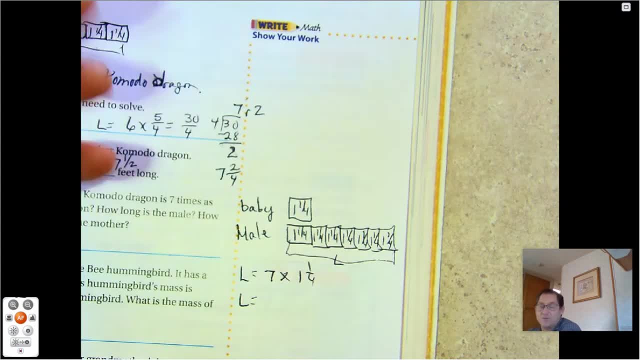 It is called an improper fraction, but we're going to say that it's an improper fraction, But we're turning it into a fraction greater than one. Okay, that's how we've been presented with it. We haven't been. we haven't named it as an improper fraction. 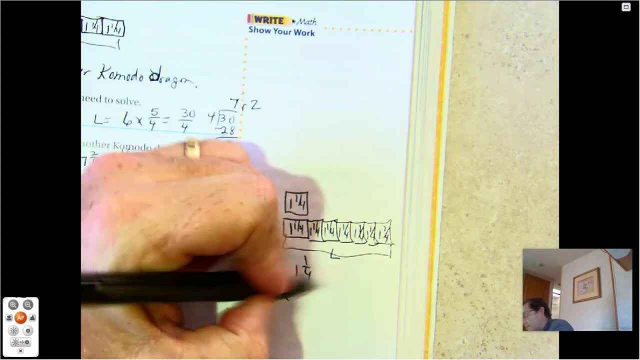 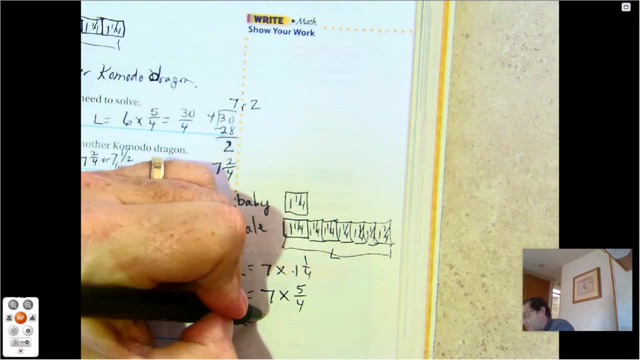 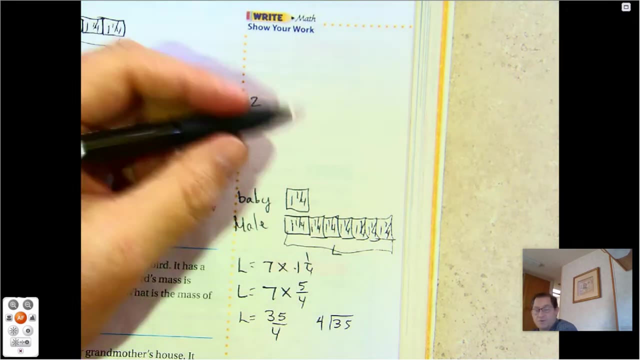 So seven times one is four plus four-fourths, So five-fourths. So the length of the male is thirty-five-fourths feet. Turn that into a mixed number. I can't share any tens with the four groups, So I'm going to share thirty-five ones. 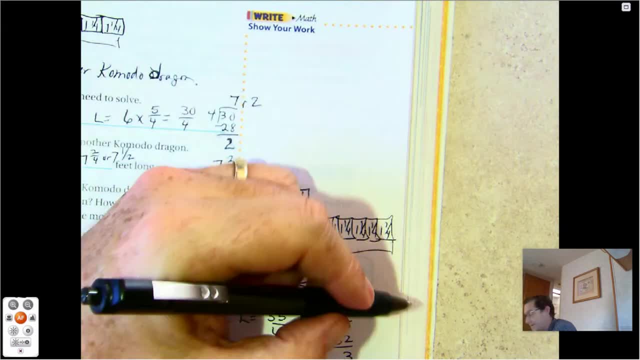 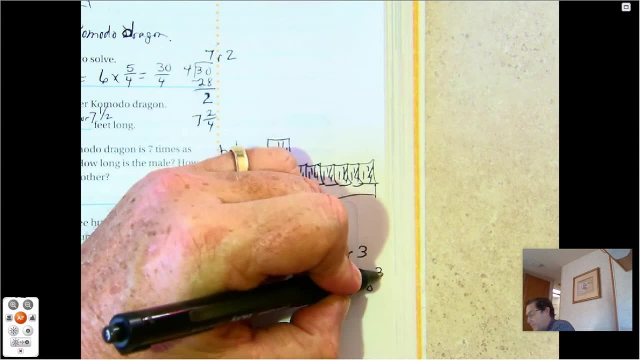 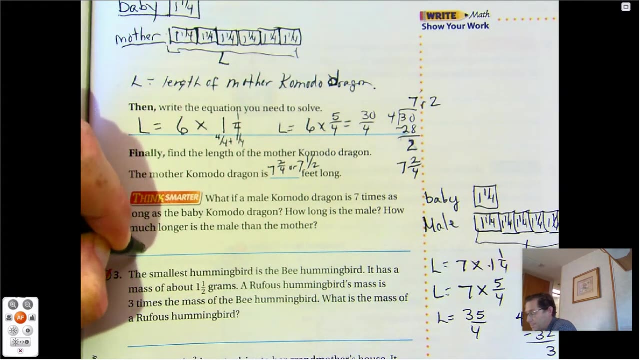 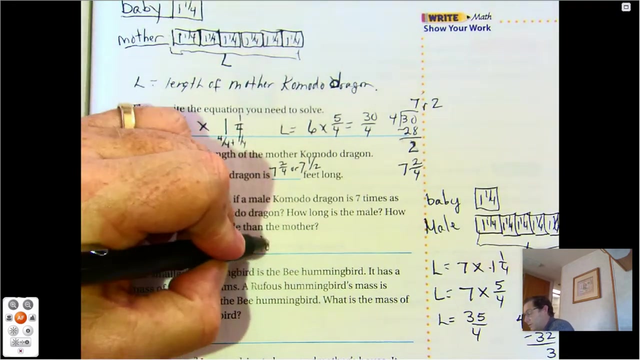 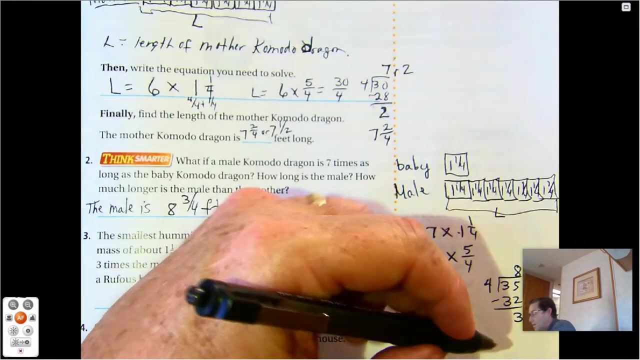 Eight times five is thirty-two ones, with a remainder of three. So eight remainder three, four, eight and three-fourths. So how long is the male Male is eight and three-fourths feet long. How much longer is the male than the female? 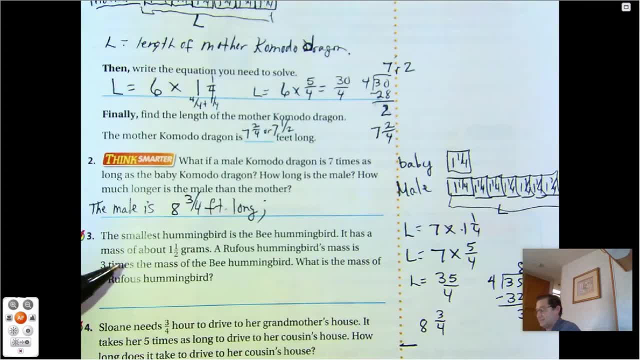 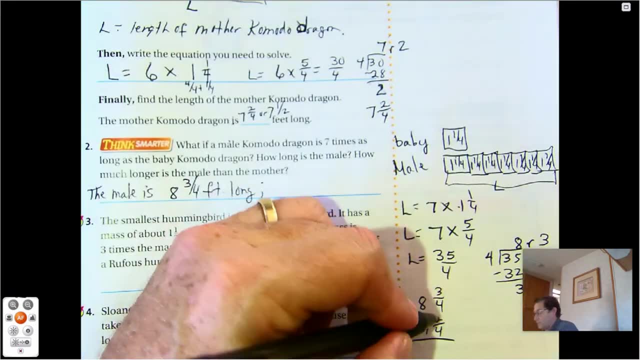 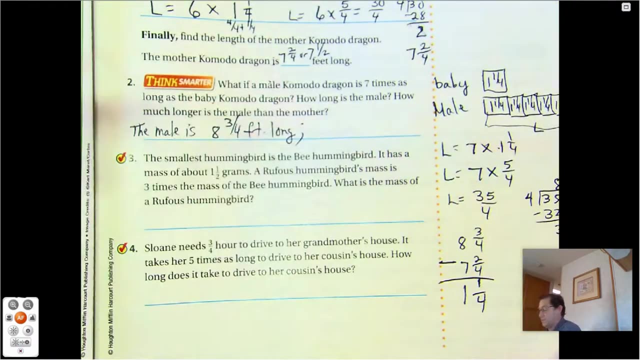 Well, the male is eight and three-fourths minus the female, which was seven and two-fourths, So three take away two is one, So one-fourth, And eight take away one is one, So one and one-fourth foot longer. 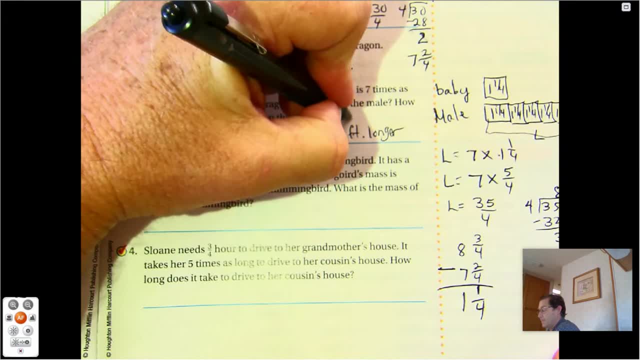 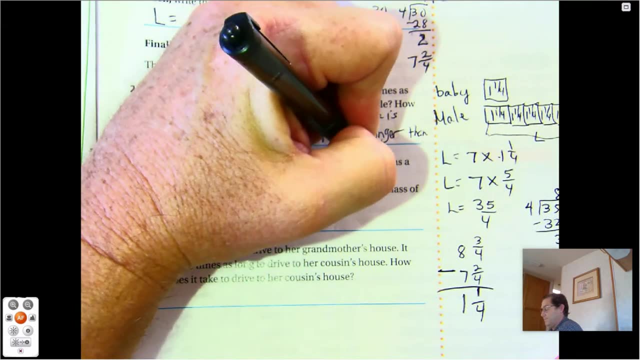 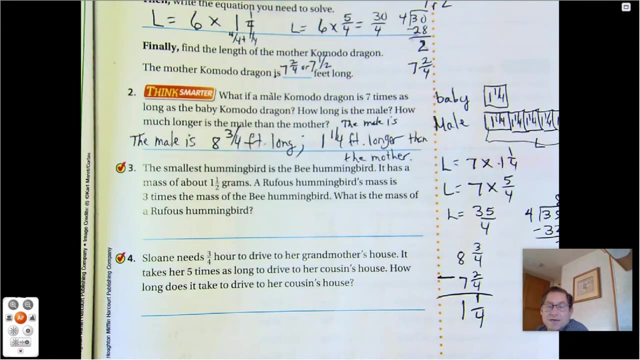 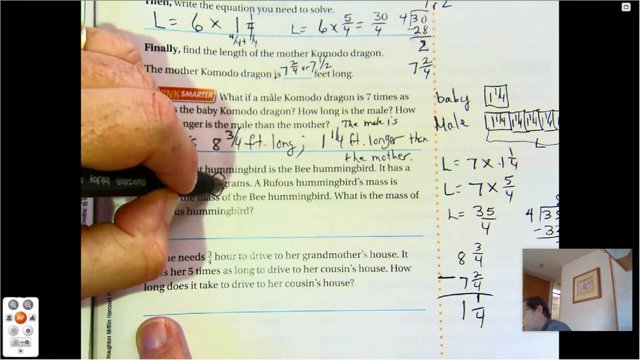 The male is one and one-fourth foot longer than the mother. All right three. The smallest hummingbird is the bee hummingbird. It has a mass of about one and a half grams. Rufus hummingbird's mass is three times the mass of the bee hummingbird. 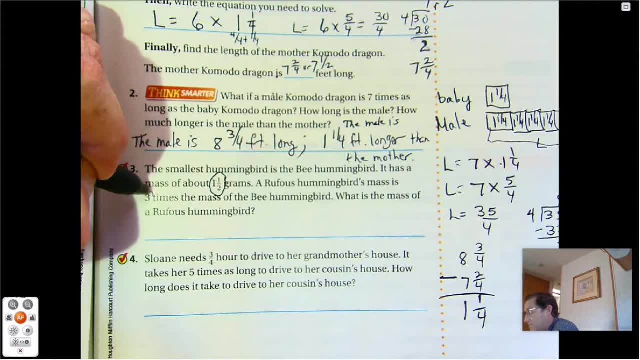 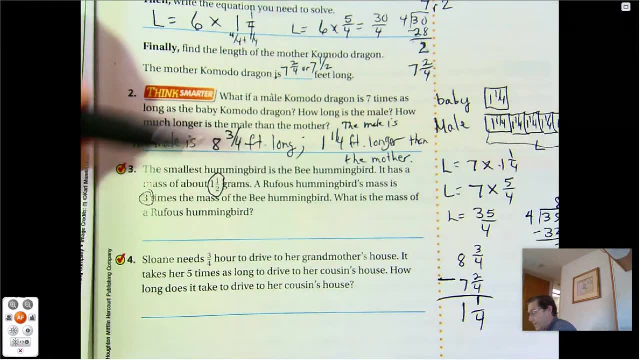 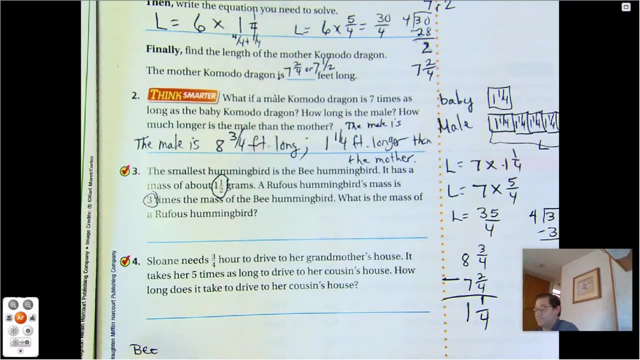 So it's about one and a half grams. So that's three times the mass of the bee hummingbird. What is the mass of a Rufus hummingbird? Okay, so we all have. I'm going to call this bee hummingbird. 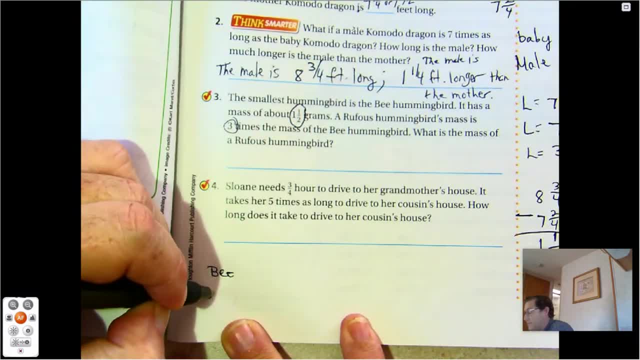 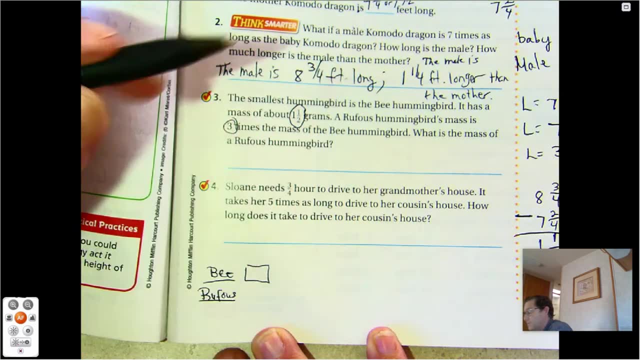 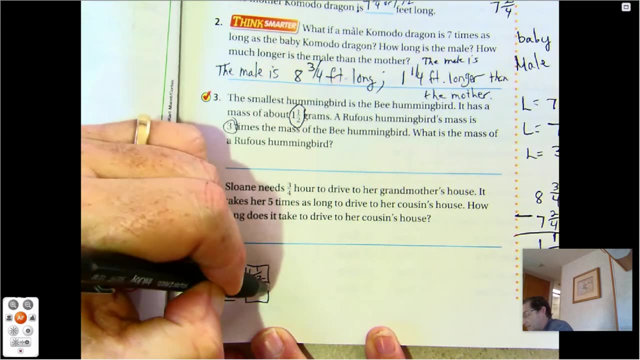 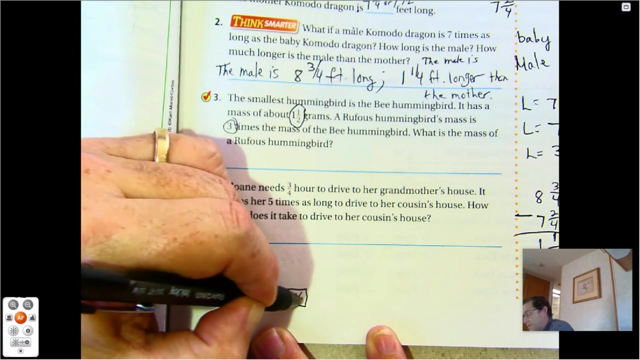 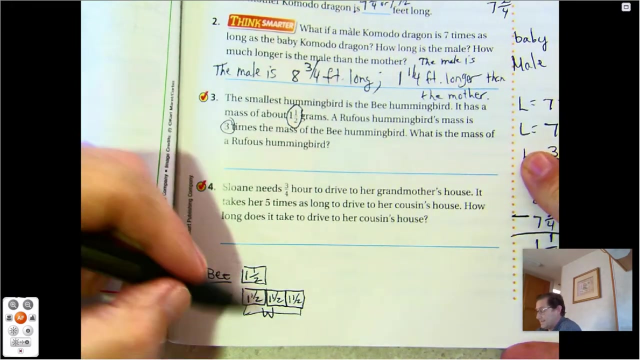 And the other one will be the Rufus hummingbird. The bee hummingbird is one and a half grams And the Rufus is one and a half grams And the Rufus is three times as much. So our equation: I can call W to be Rufus's weight. 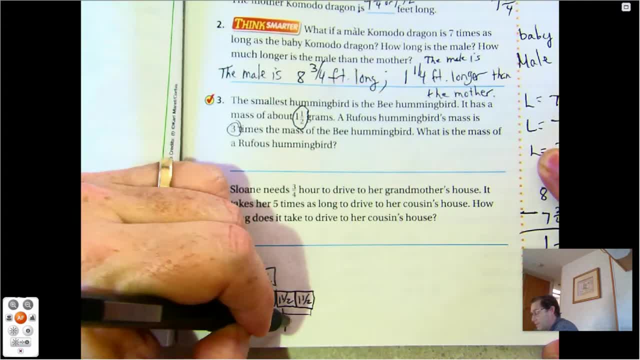 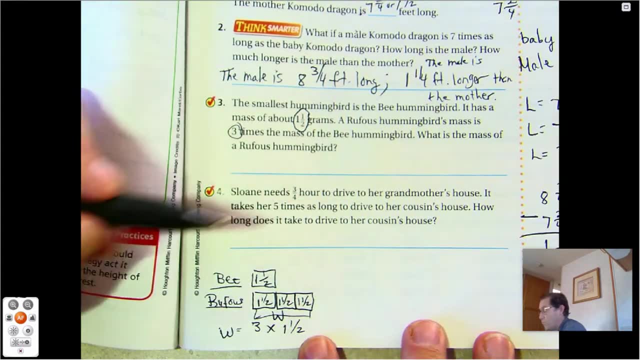 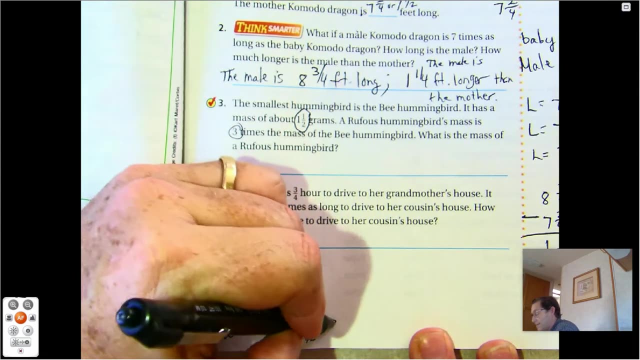 So W equals three times one and one-half. We're going to change one and a half into a fraction that's greater than one. How many parts are in this one? Two halves plus one-half. So we have three times three halves, which is nine halves. 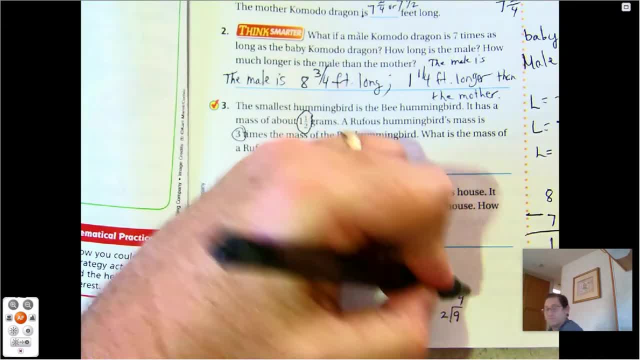 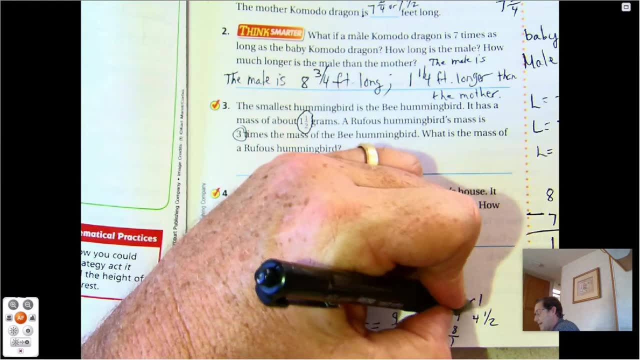 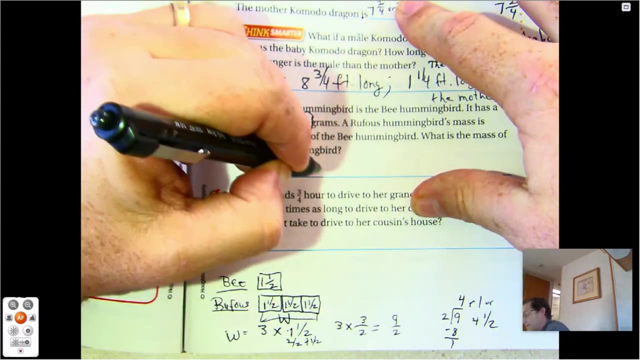 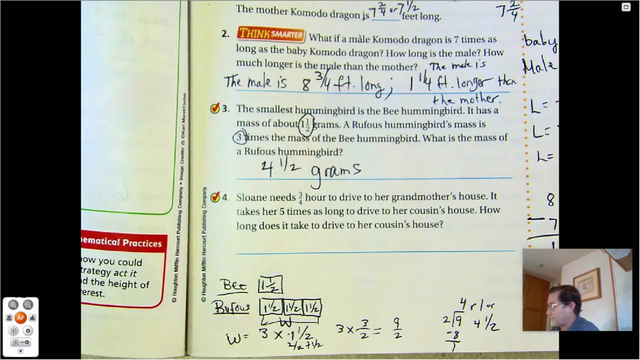 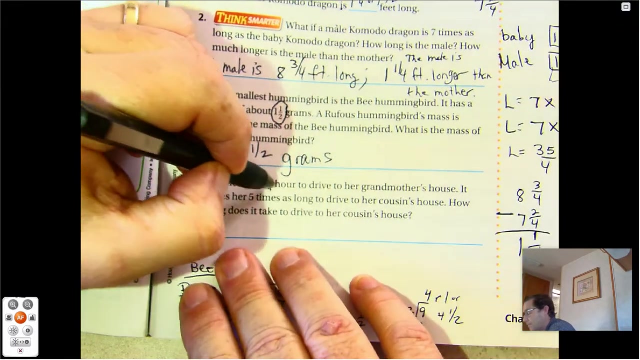 Nine divided by two, I can put four into each group, with a remainder of one, So four and one-half. What is the mass? It's four and one-half grams. Number four: Sloane needs three-fourths hour to drive to her grandmother's house. 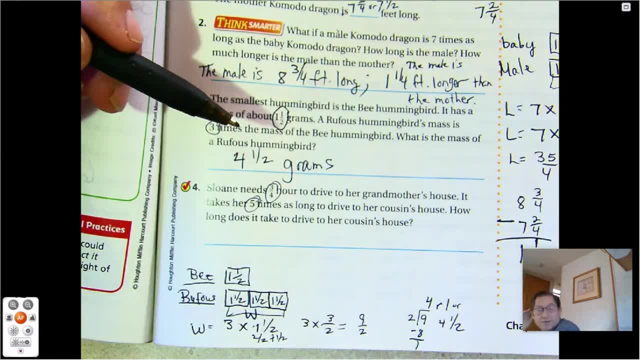 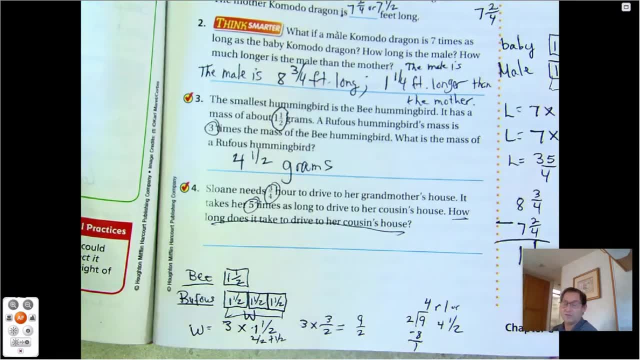 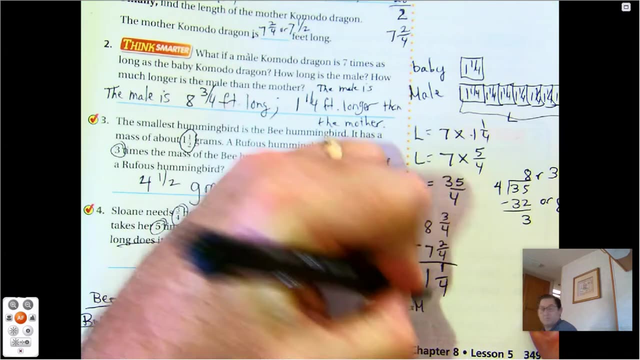 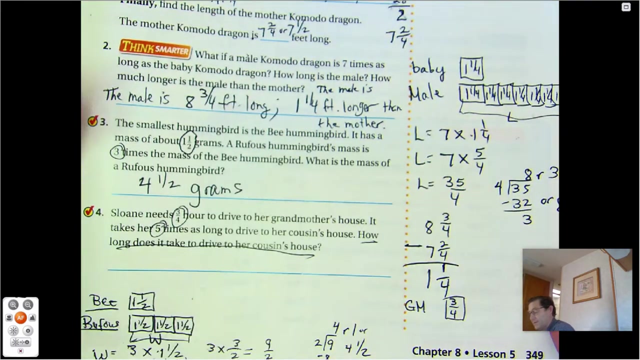 It takes her five times as long to drive to her cousin's house. How long does it take to drive to her cousin's house? Okay, again, we can draw a picture for this. We can say grandma three-fourths And cousin five times. 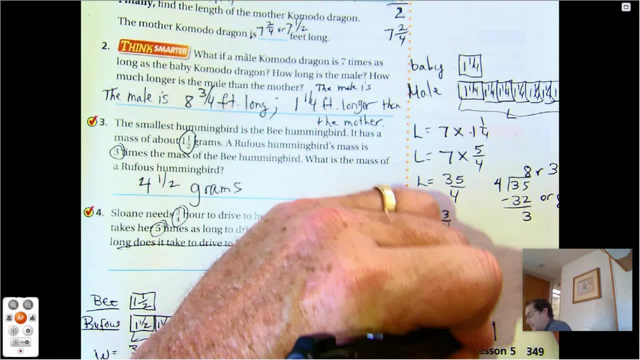 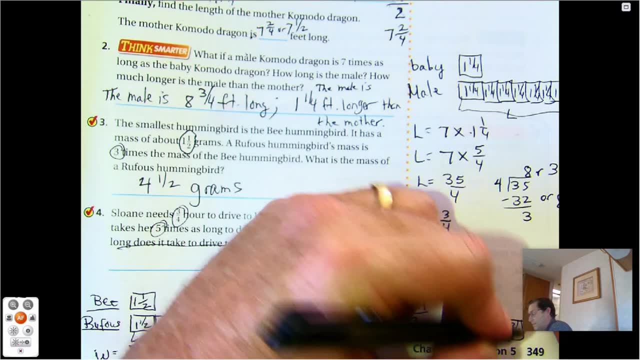 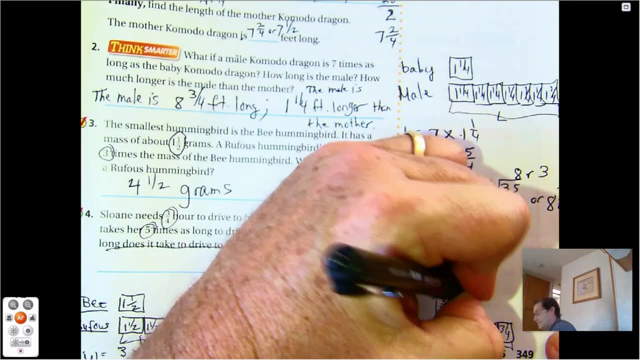 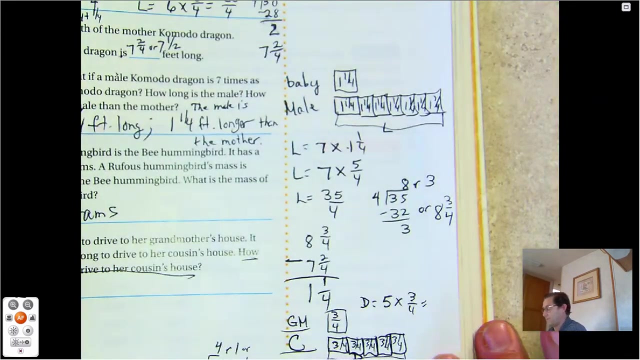 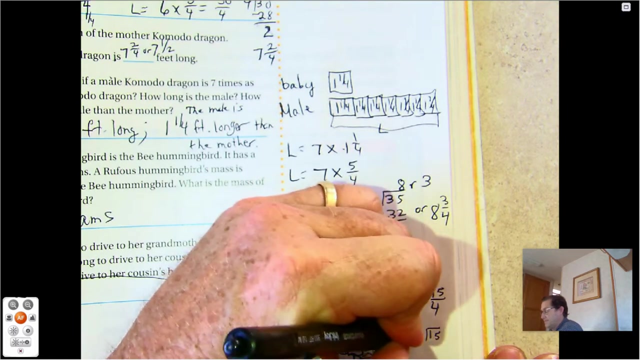 One, two, three, four, five. We can call that d for distance. So d equals five times three-fourths. Well, five times three-fourths is fifteen-fourths, What is fifteen divided by four, Because we have to turn it back into a mixed number. 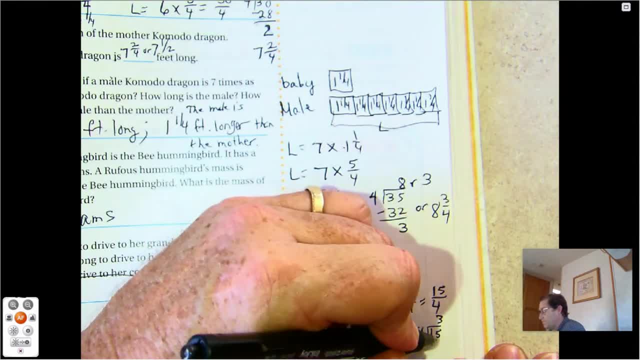 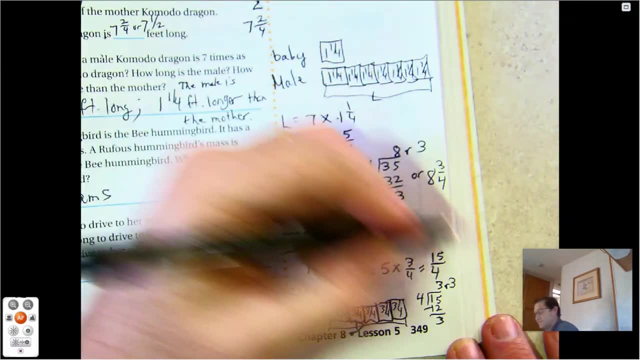 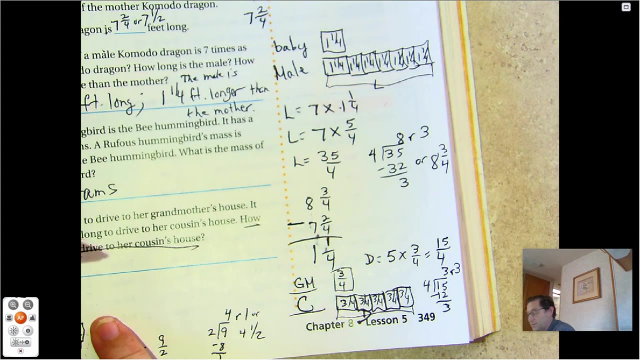 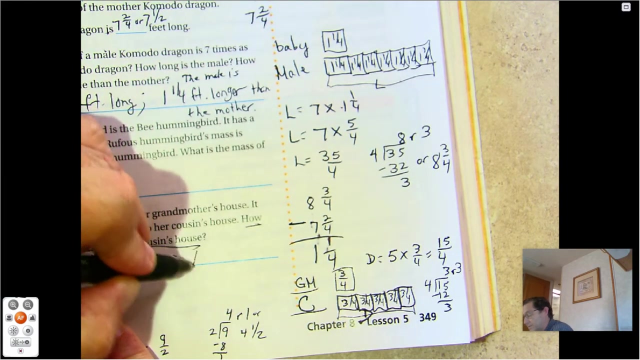 Four times three is twelve, with a left-over. Four times three is twelve with a left-over Three ones. So three and three-fourths Takes three and three-fourths hours to drive to the cousin's house, So three and three-fourths. 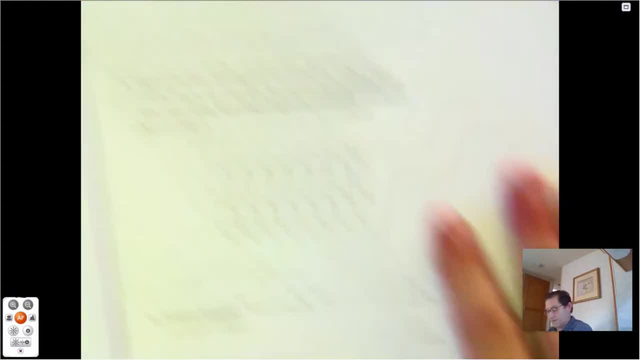 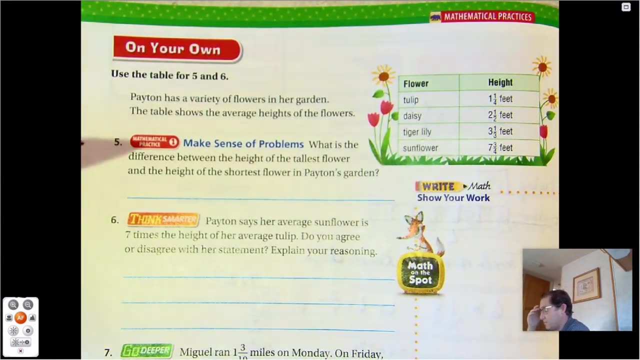 Takes three and three-fourths hours to drive to the cousin's house. Okay, page 330.. Use the table for numbers five and six. Okay, so let's look at our table. Make sure we understand what the table is trying to tell us. 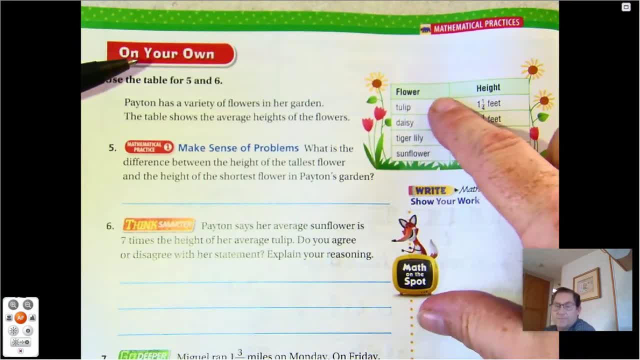 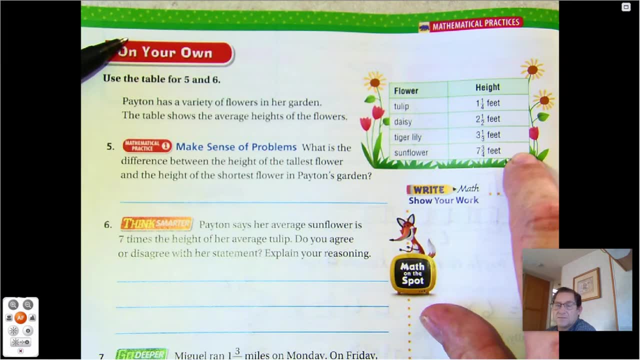 Make sure we understand what the table is trying to tell us. So we have a heading called flower, And so these are four different types of flowers And these are the height of the different flowers. Okay, I see that the smallest flower here listed is the tulip. 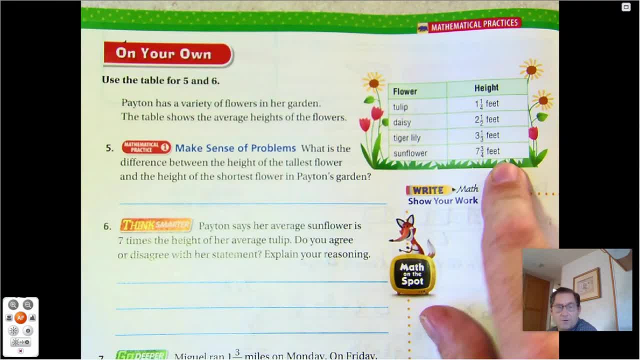 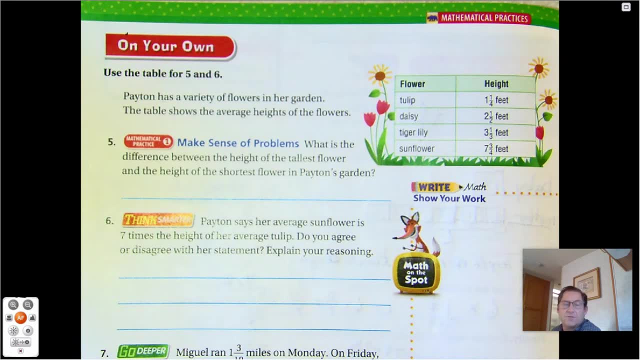 I see that the smallest flower here listed is the tulip and the largest flower is the sunflower. Alright, So Peyton has a variety of flowers in her garden. The table shows the average heights of the flowers. Okay, What is the difference between the height of the tallest flower? 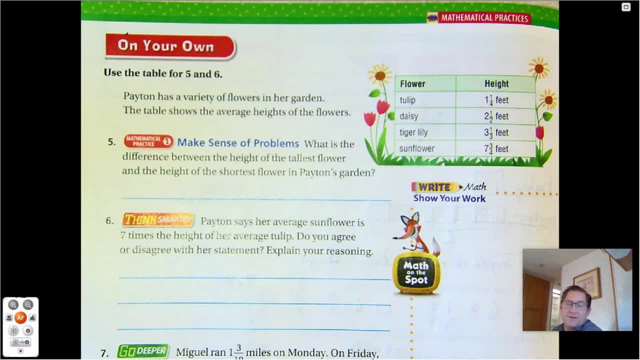 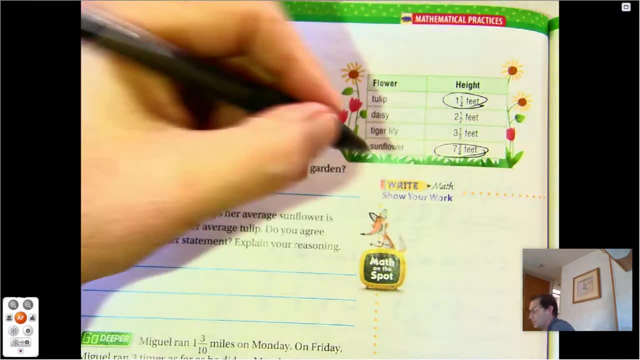 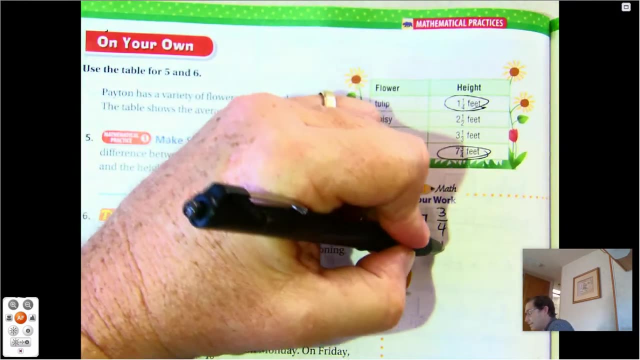 What is the difference between the height of the tallest flower and the height of the shortest flower? and the height of the shortest flower? Okay, So the tulip is the shortest and the tallest is the sunflower. Seven and three-fourths: take away one and one-fourth. 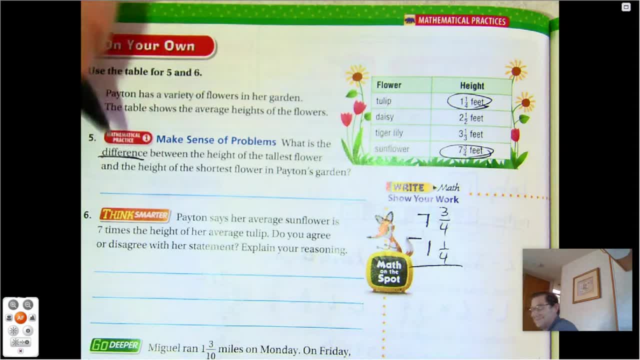 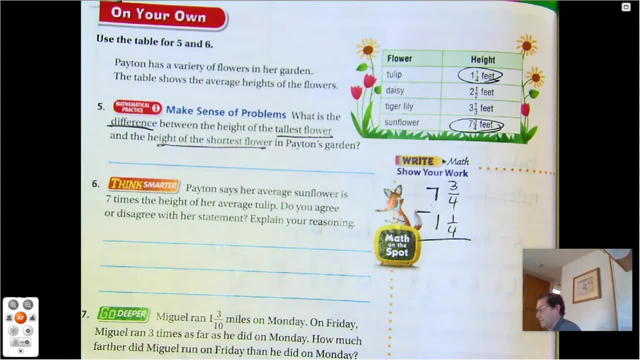 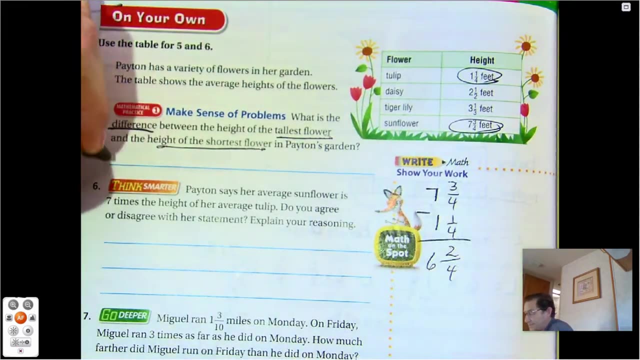 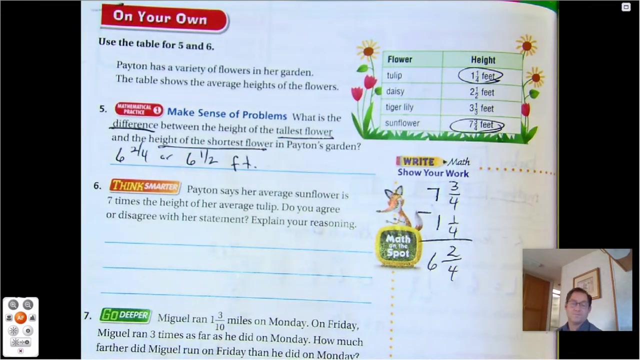 It wants to know what is the difference between the tallest and the shortest. Okay, differences of track Three. take away, one is two, so two-fourths. So six and two-fourths feet, or six and one-half Eight feet is the difference. 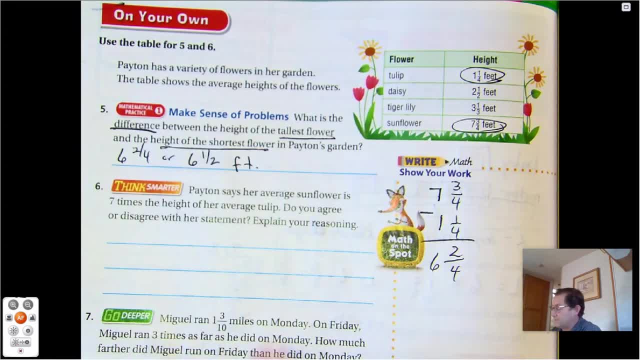 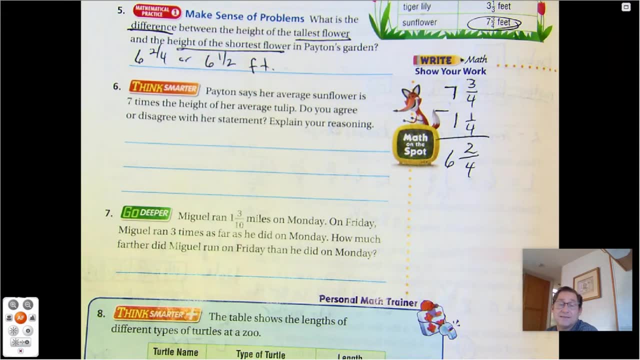 Okay, remember, half of four is two, so it's simplified would be six and a half. Number six: Peyton says her average sunflower is seven times the height of her average tulip. Do you agree or disagree with her statement and explain your reasoning? 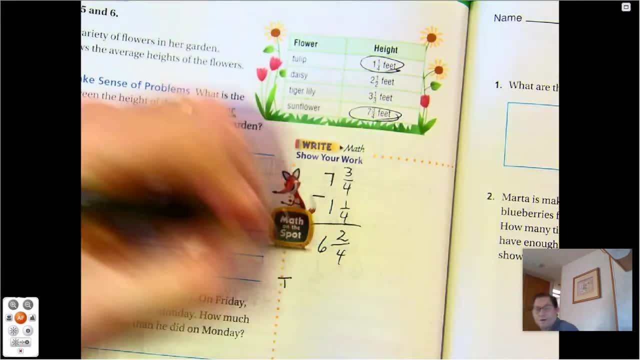 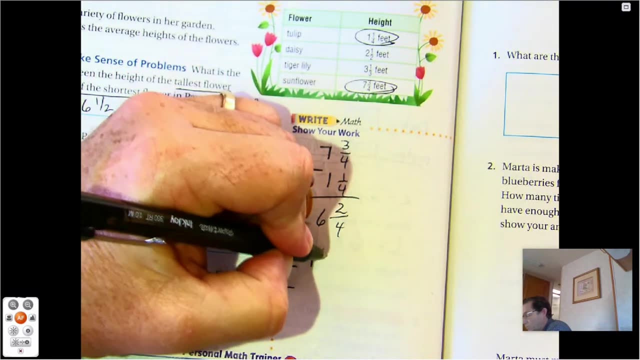 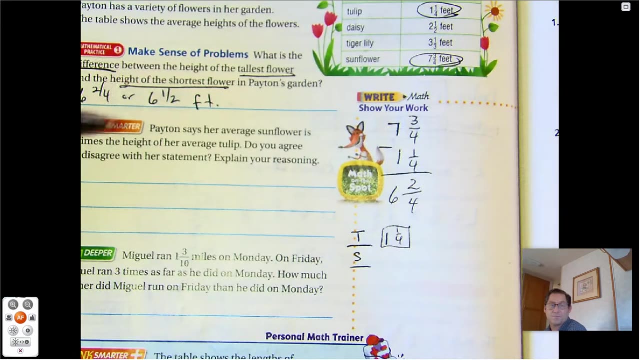 Okay, so tulip, I'm going to write T for tulip and S for sunflower. The tulip is one and one-fourth feet. The sunflower, she's saying, is seven times. Okay, her claim is that it's seven times as much. 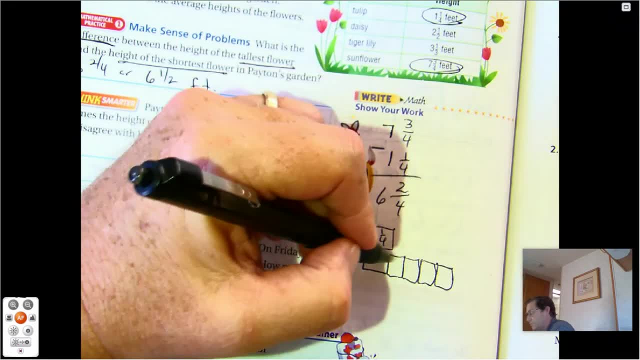 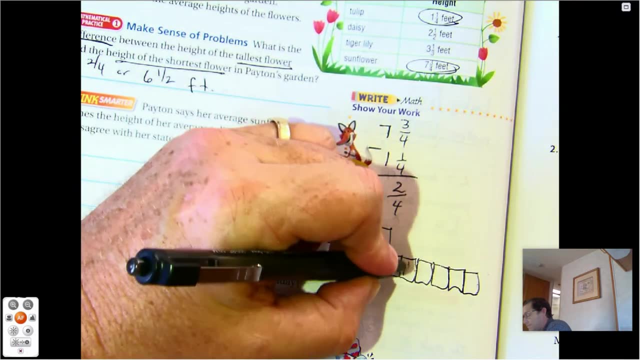 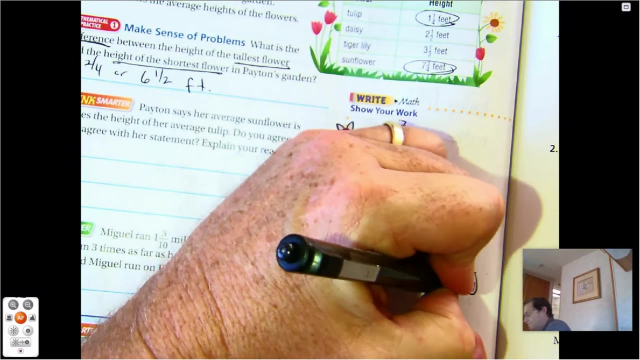 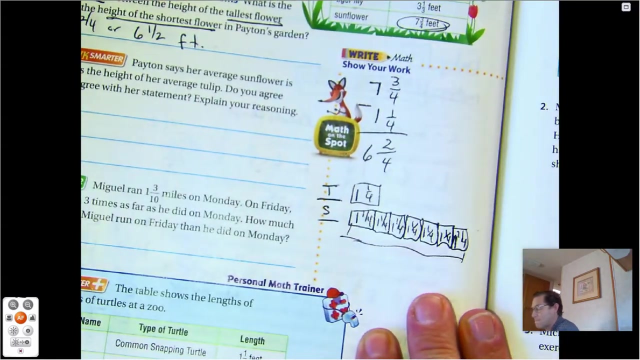 So, if that's true, we can draw a model to show that Two, four, five, six, seven, And every one of them is one and one-fourth. We'll call this H the height. let H equal the height of the sunflower. 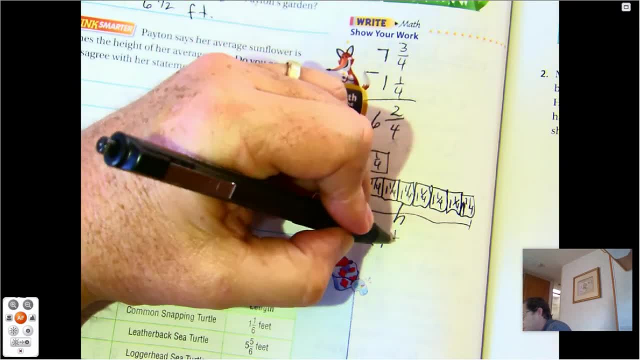 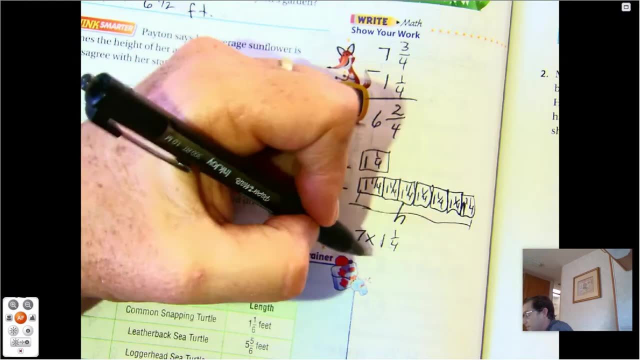 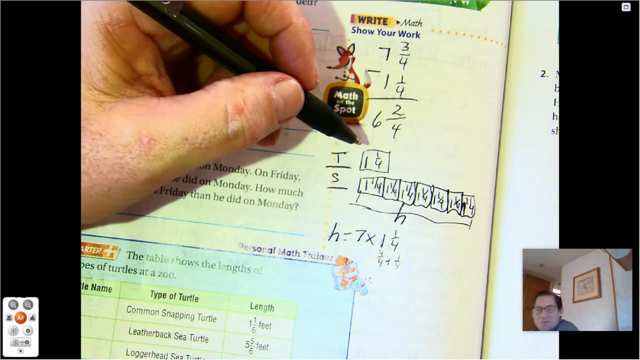 So H equals seven times one and one-fourth. Well, what is one and one-fourth? as a mixed, as a fraction greater than one? Well, in the one there's four and four parts, Four and four, Four out of four parts, to equal one plus the leftover one-fourth. 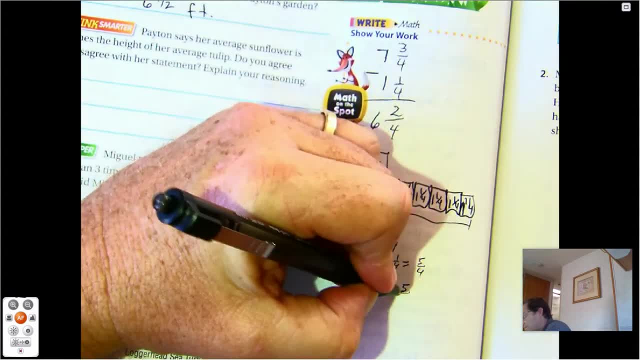 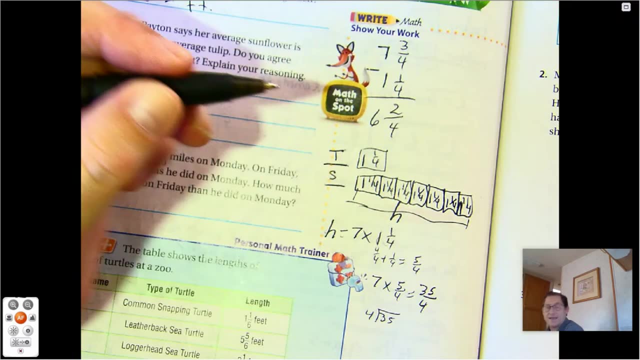 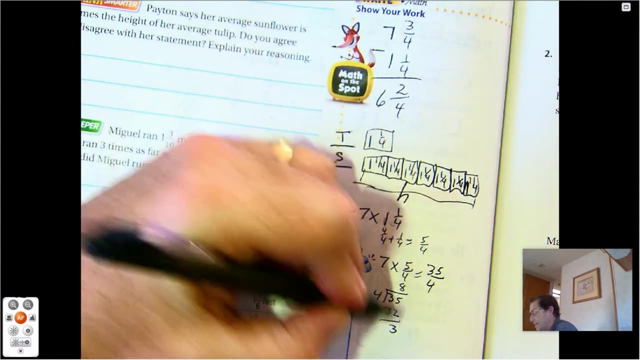 So that's five-fourths. So seven times five-fourths gives me 35-fourths. Turn that back into a mixed number. How many fours can I divide into 35? Eight With a remainder of three. So eight remainder of three, or eight and three. 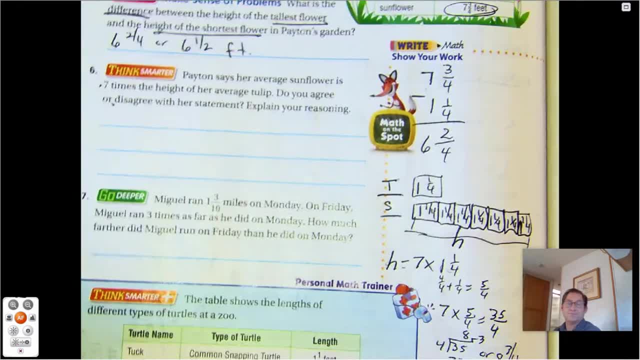 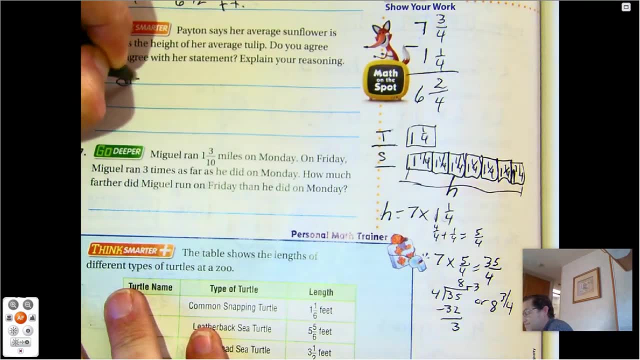 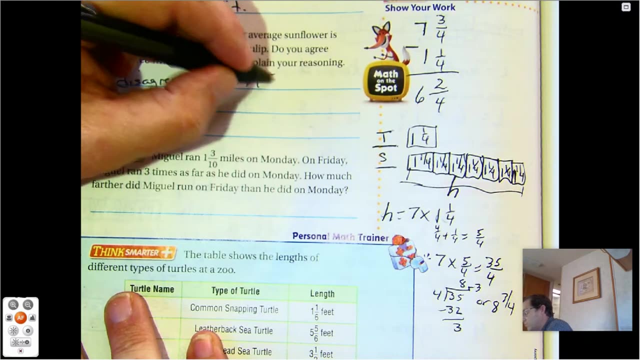 Eight-fourths. So now back to our question. Peyton says the average sunflower is seven times the height. I guess I would disagree. I would disagree: Seven times one and one-fourth equals eight and three-fourths, Which is more. 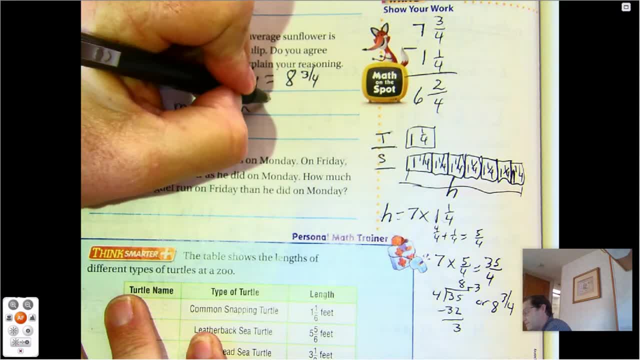 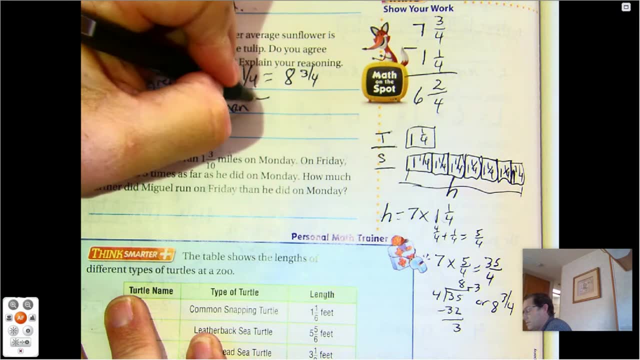 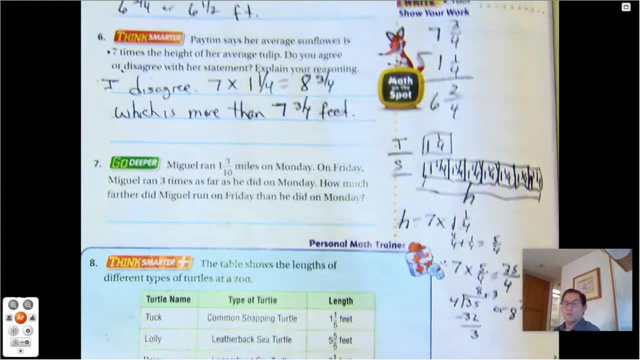 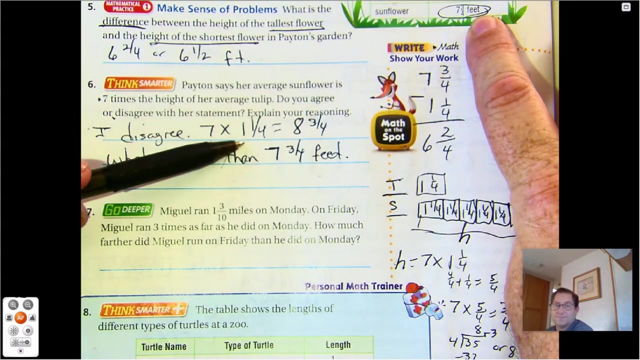 More, More than seven and three-fourths feet. Okay, So remember that the height of the flower is seven and three-fourths feet. She said that it was seven times. Well, if I multiply seven times one and one-fourth, I get eight and three-fourths. 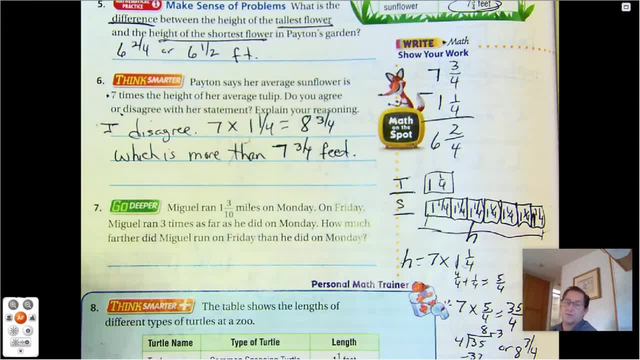 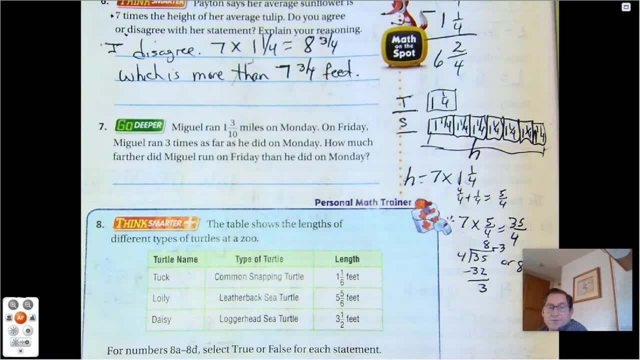 So I'm actually more than seven and three-fourths feet. So it's more than seven and one-fourth, More than seven times Number seven. Miguel ran one and three-tenths miles on Monday. On Friday, he ran three times as far. 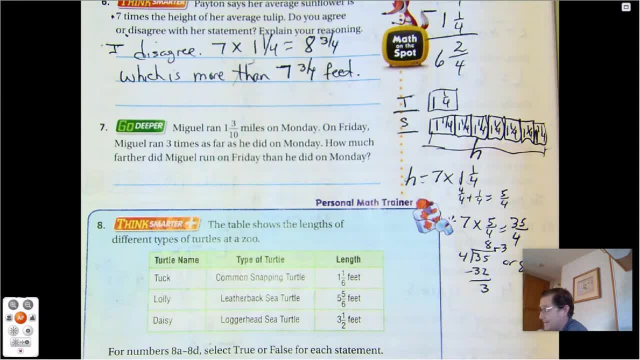 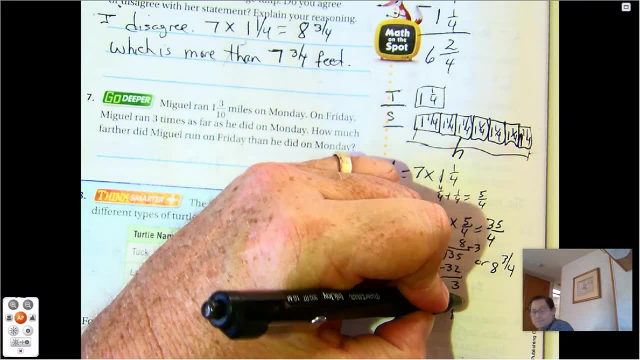 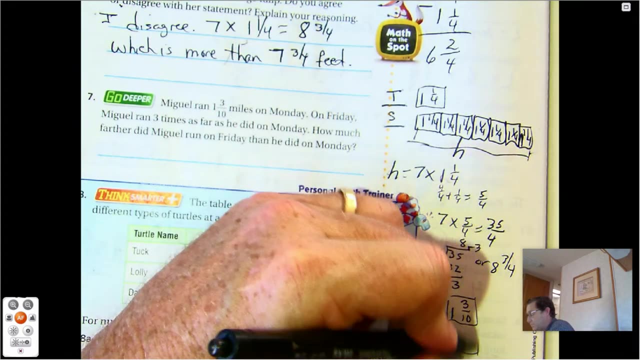 How much farther did Miguel run on Friday than he did on Monday? All right, So we can again draw a diagram: Monday one and three-tenths. Friday he did three times as much. So one, two, three. 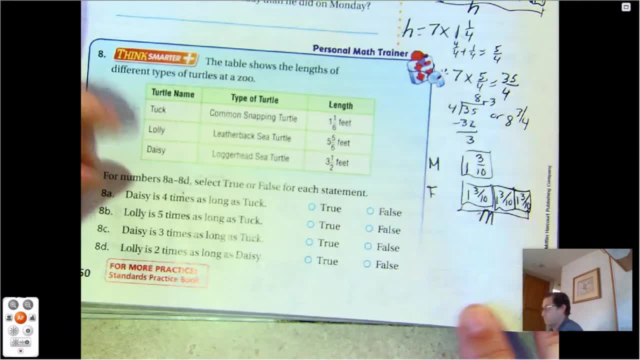 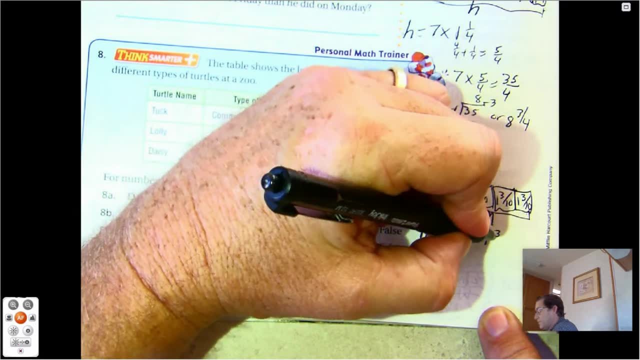 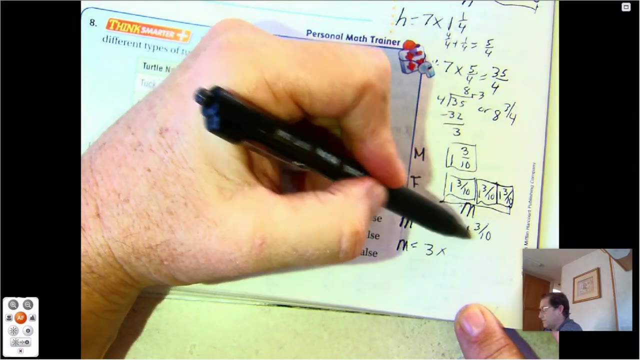 We can just call that miles. So how far did he run on Friday? Miles equals three times one and three-tenths, So three times In every one hole in this problem. it's ten-tenths plus the leftover three-tenths. 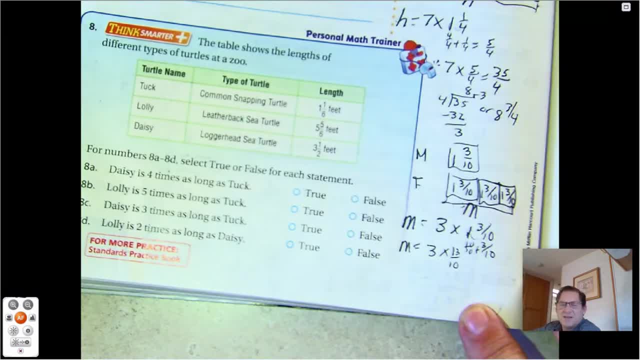 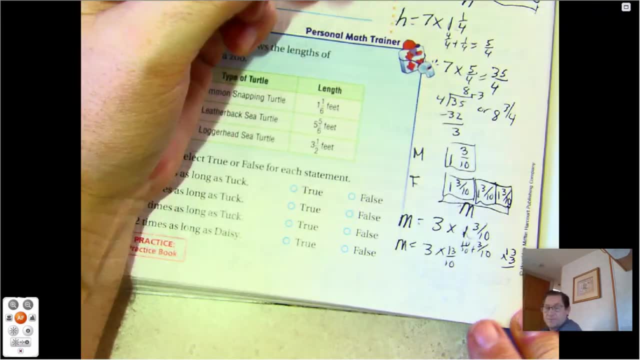 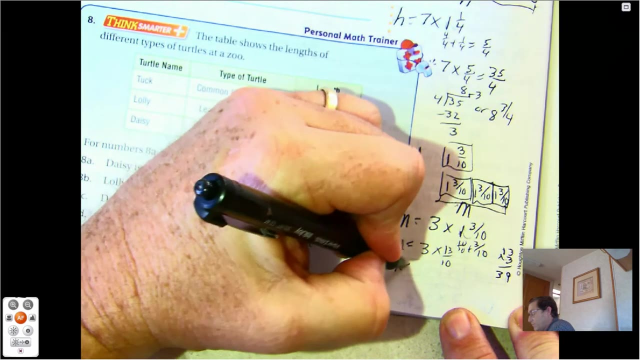 So we get 13-tenths. So what's three times 13?? Well, we know how to do this: Three times three-ones is nine-ones, And three times ten is 30.. So 39.. So 39-tenths. 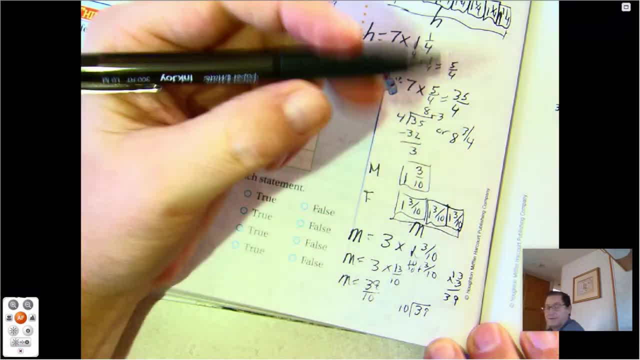 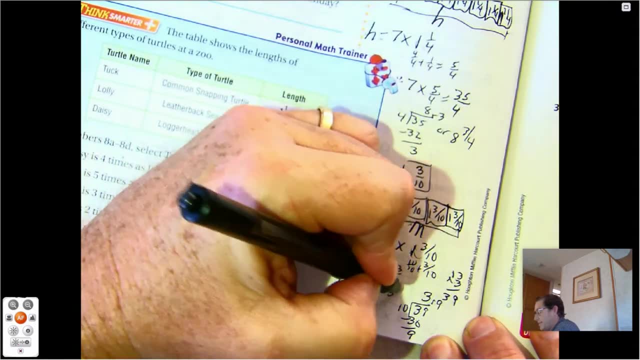 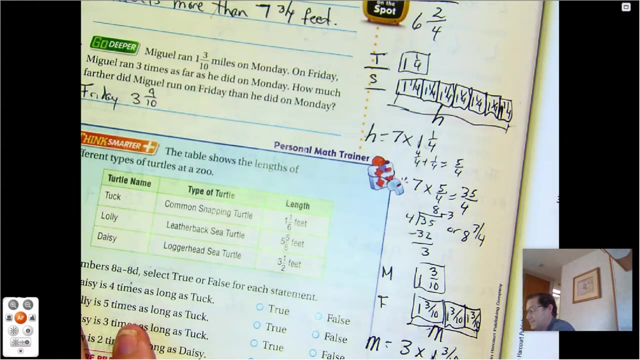 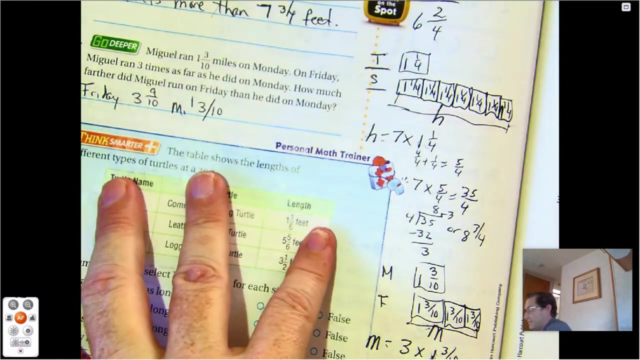 So how many tens Can be shared with 39.. Three With a remainder of nine. So three and nine-tenths, Friday, three and nine-tenths, Monday, one and three-tenths. So the difference, how much farther we need to subtract? 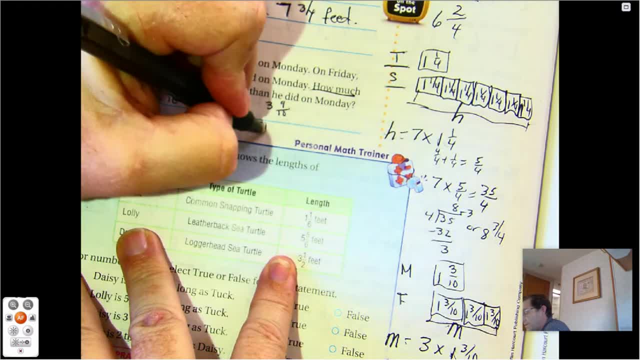 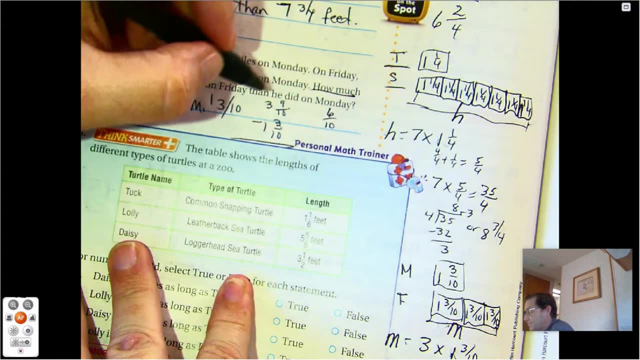 So three and nine-tenths take away one and three-tenths. Nine take away three is six-tenths. Three take away, one is two. So two and six-tenths. I know that two and six are both even. 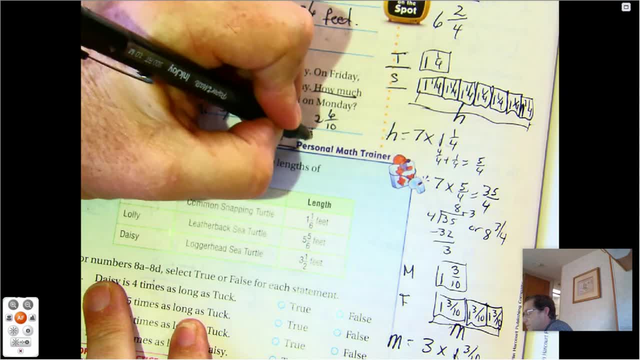 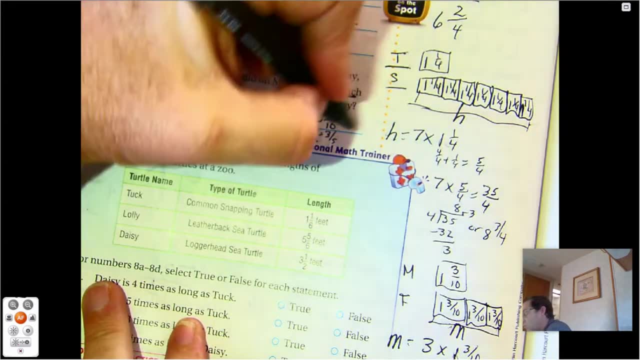 So I know I can divide them both by two, So two and six-tenths, or two and three-fifths. So I know I can divide them both by two, So two and six-tenths, or two and three-fifths. 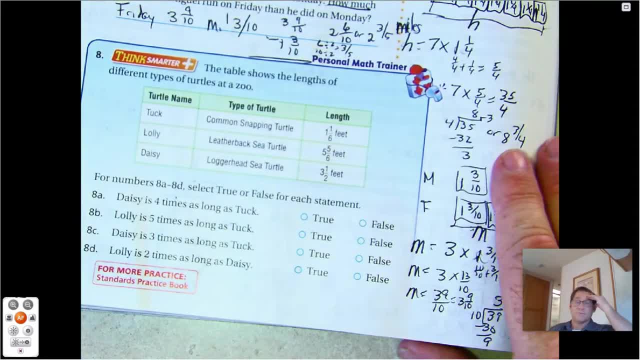 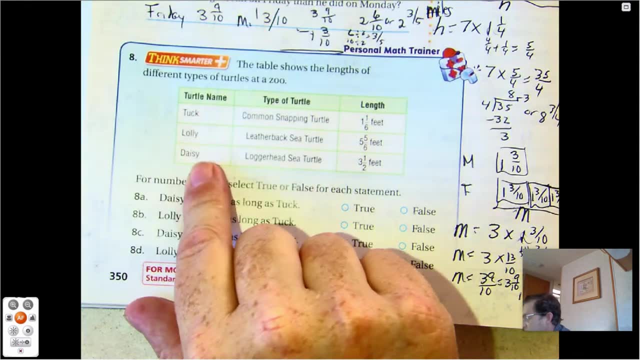 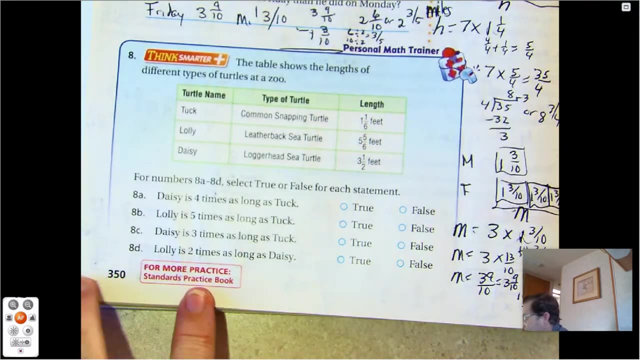 Miles further. Number eight: The table shows the length of different types of turtles at a zoo. Alright, So we have three different turtles. These are the type of turtles and their lengths. Okay, so For 8a through 8d, select true or false for each statement. 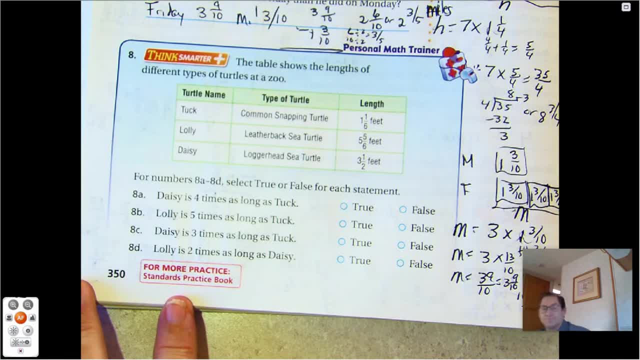 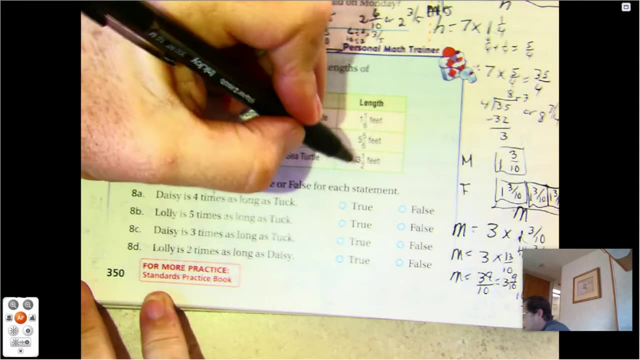 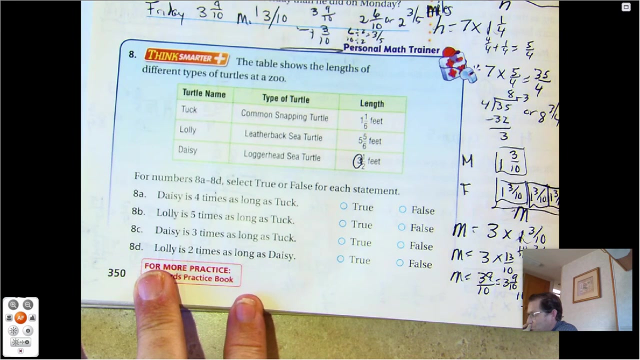 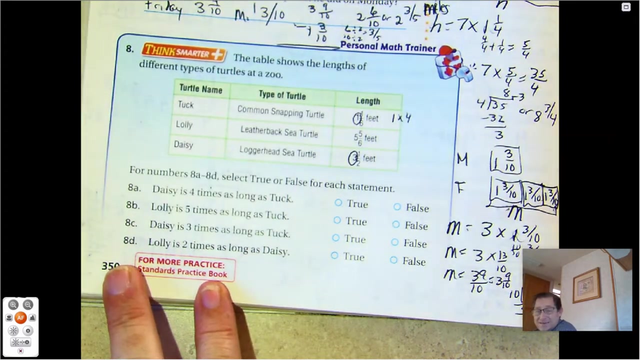 Daisy is four times as long as Tuck. Daisy is four times Well, we can use common sense on that one. so Daisy is 3 feet, Tuck is 1 and 1 sixth. so if I just multiplied 1 times 4, I'd get 4 feet. so Daisy's not that long, so false. 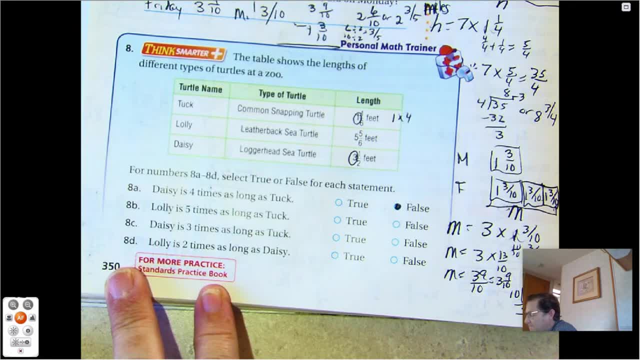 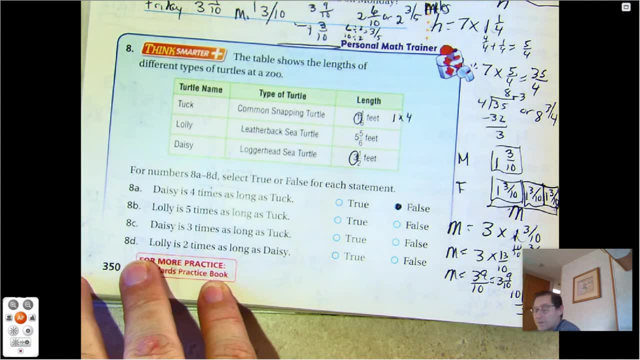 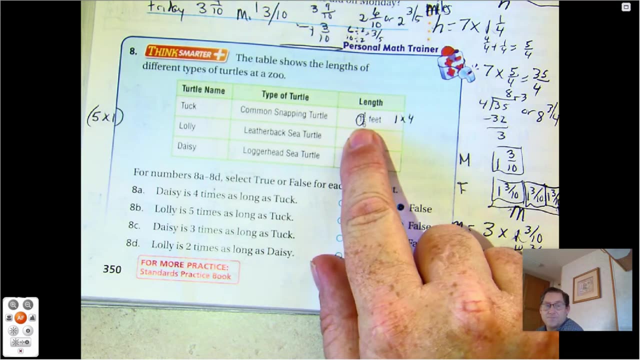 Okay, Lolly is 5 times as long as Tuck. well, that's possible, okay. so let's see 5 times 1, okay, so we're going to split this up 5 times 1 plus 5 times 1. sixth, okay, remember.